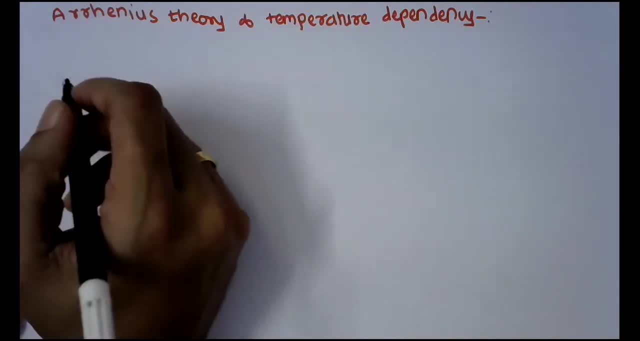 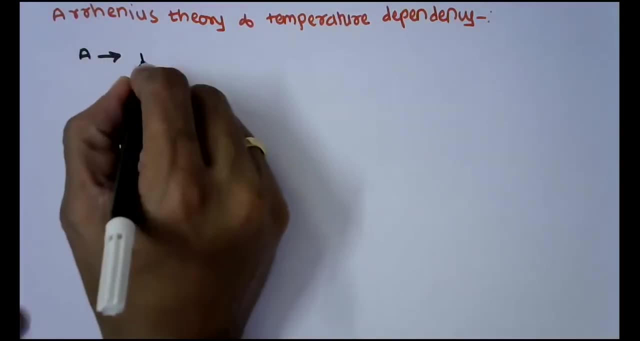 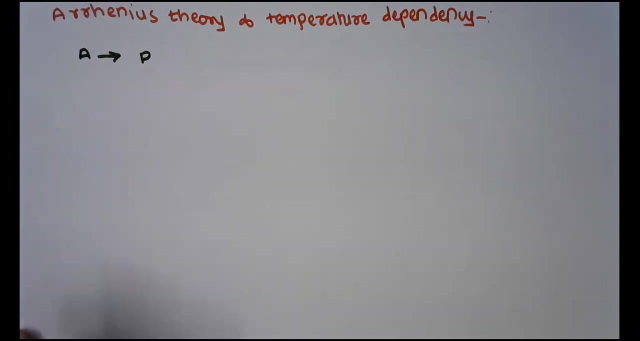 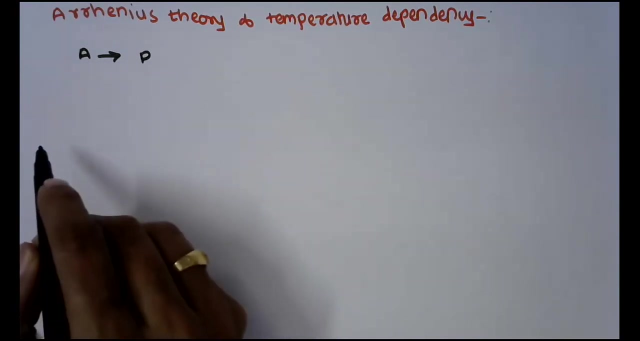 the reaction of a reaction A gives P. Now the rate at which this reactant A will be converted into P is the function of concentration of reactant A and the temperature. Now suppose, if we assume concentration of reactant A constant, 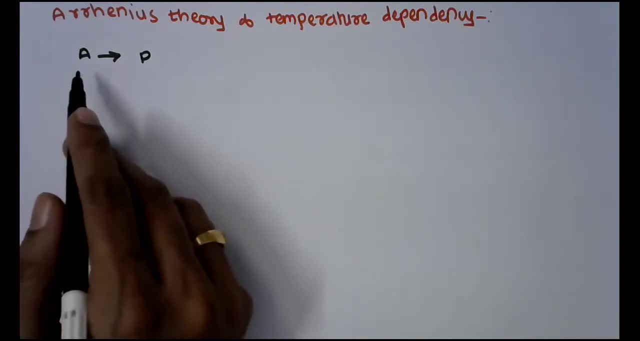 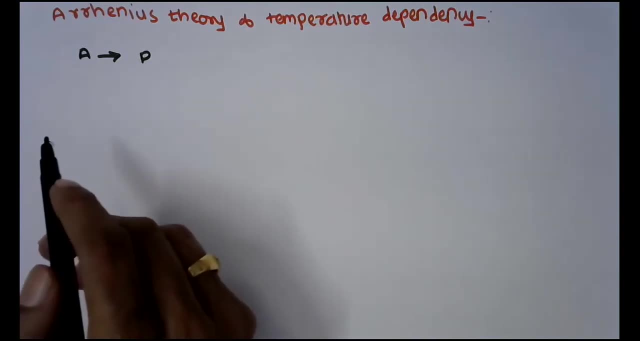 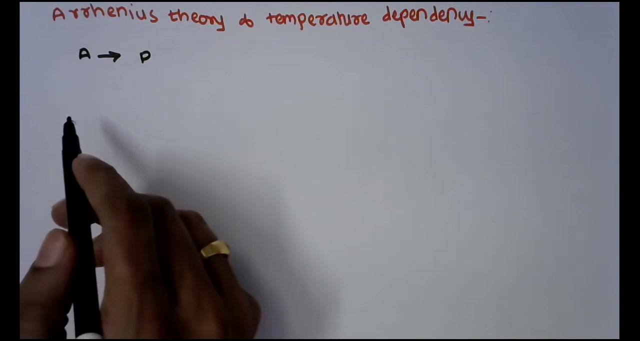 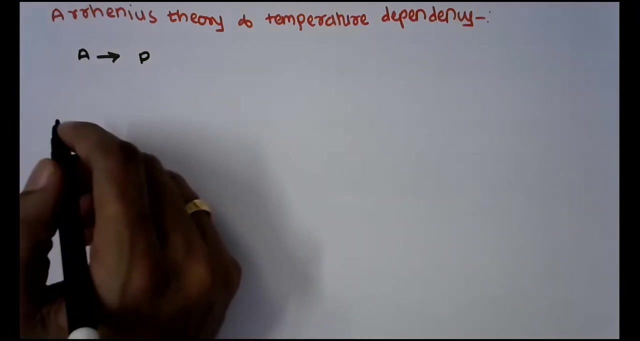 And if we carry out the reaction or experimental trial at a various temperature or at a different temperature, then the ratio of rate constant will provide the accelerating and information about accelerating effect of temperature. Now, before we proceed further, we are going to execute a equivalence. Therefore, let us try to understand that some範 trees. 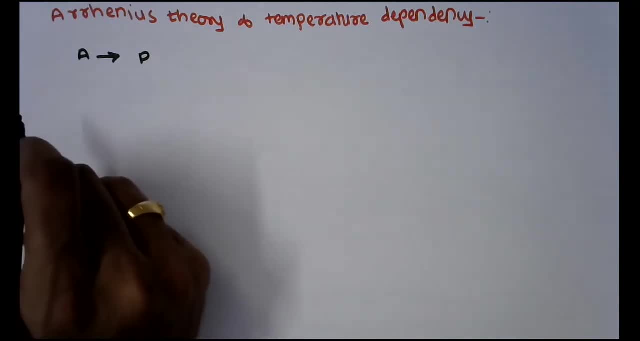 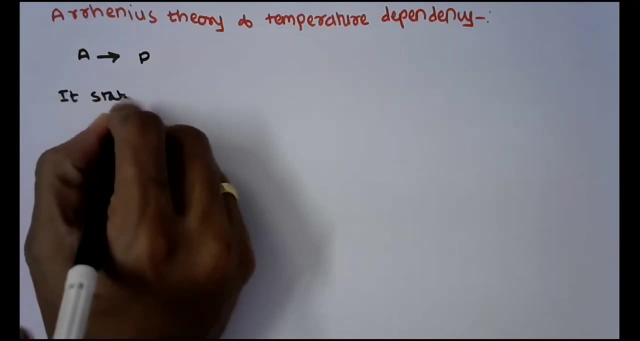 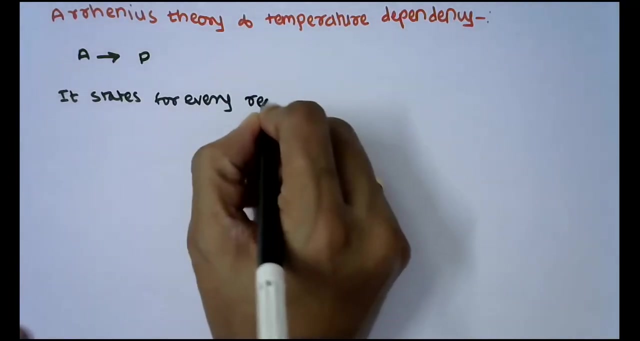 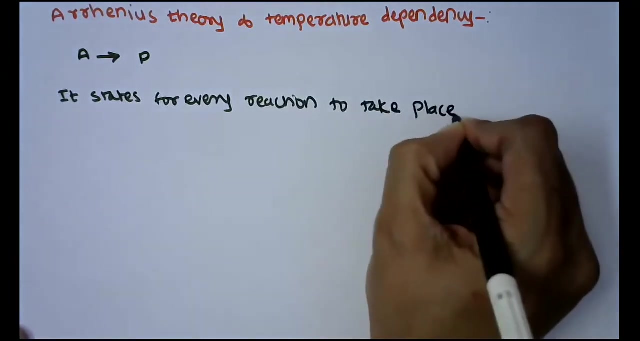 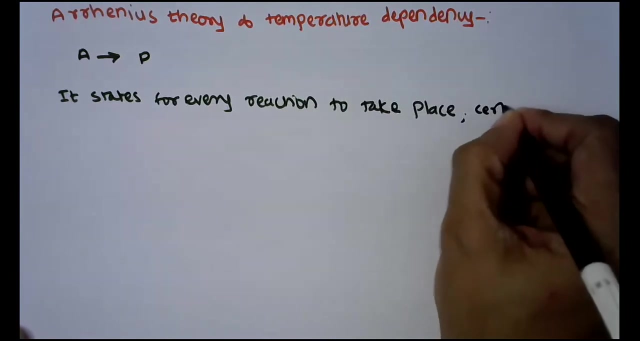 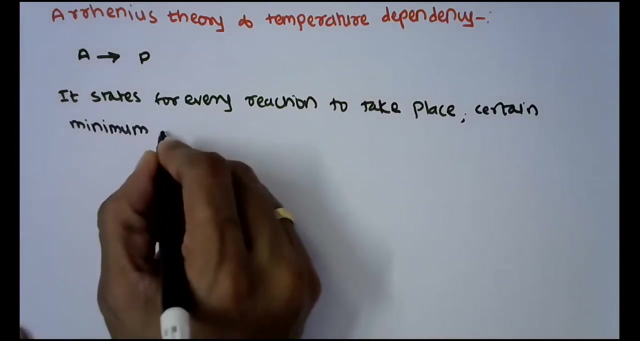 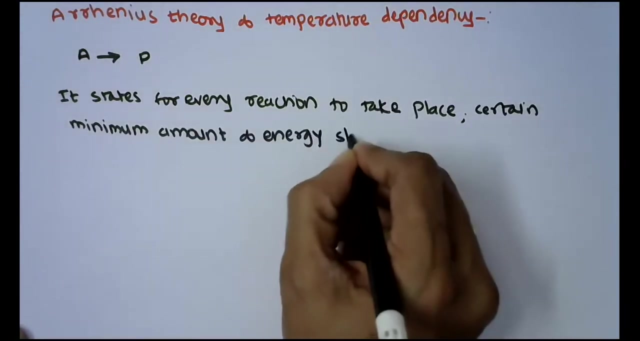 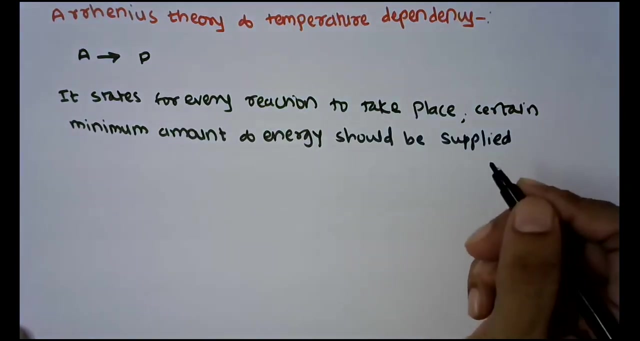 do not do that. Salient features of theory: Arrhenius theory. Video 2: So it's takes. it states viewers, dialogue 5 For a All intoxicated object. it speaks abut every reaction to take place. Video D: certain minimum amount of energy should be supplied. 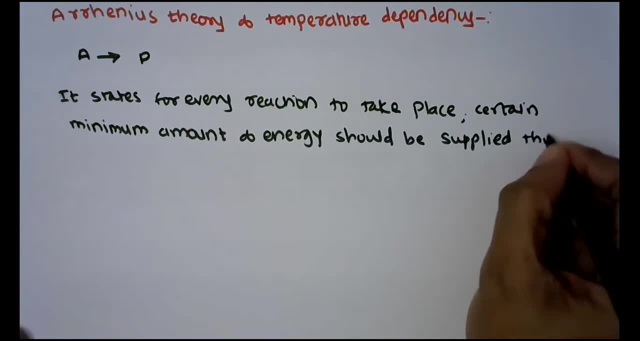 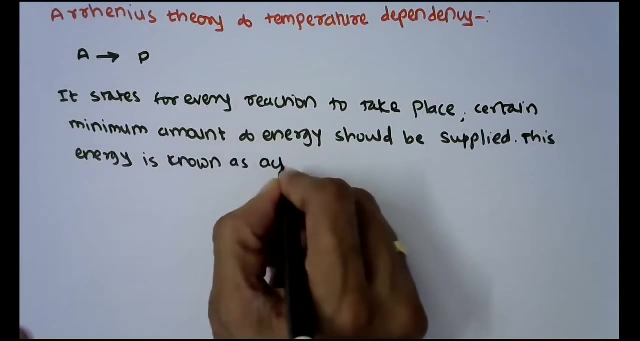 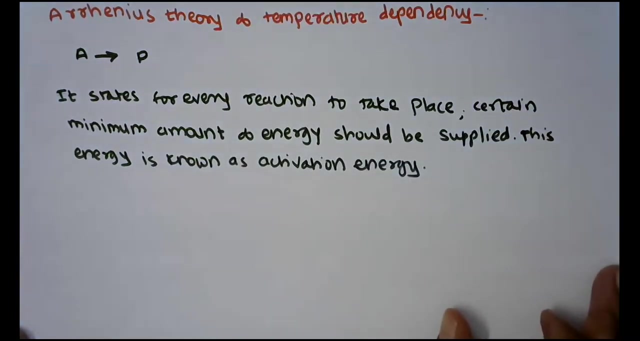 This energy is known as activation energy, So for a particular reaction, Since the activation energy is the energy required for making or breaking of the bonds or for the rearrangement of the bonds, thereby the formation or the conversion of reactant into product. as it is a compound specific, it will remain constant. 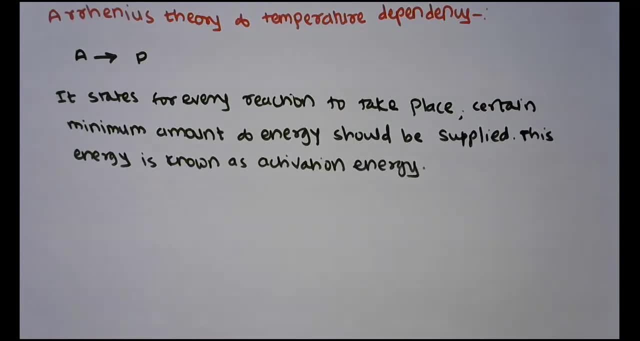 However, the rate of reaction will be affected by the temperature at which the reaction is carried out Now. so, as per the Arrhenius theory, certain minimum amount of the energy is to be supplied in order to initiate the reaction Now. and once that energy is supplied, the collision between the molecules, the reaction. 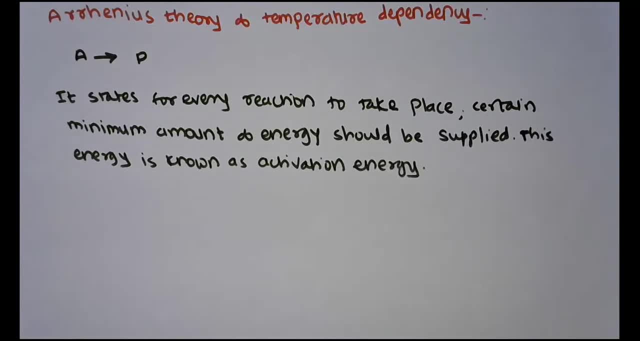 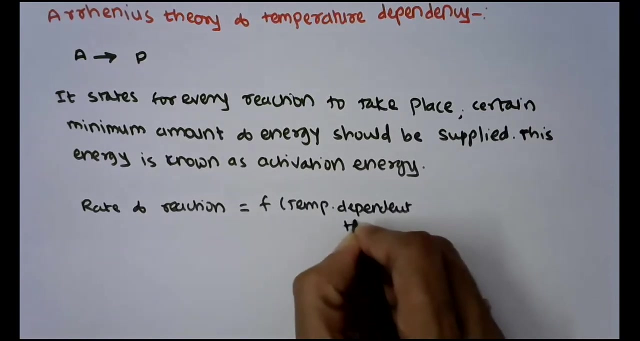 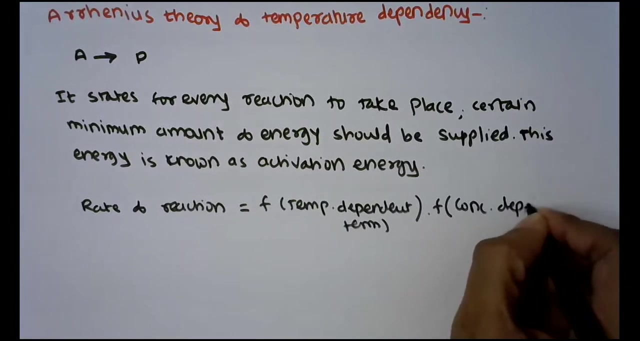 will occur If they are energetic, and they will be because you are supplying certain minimum amount of energy, the reaction will occur. Now we have studied that rate of reaction is function of temperature dependent term and function of concentration dependent term. The rate of reaction is the function of temperature dependent term and function of concentration. 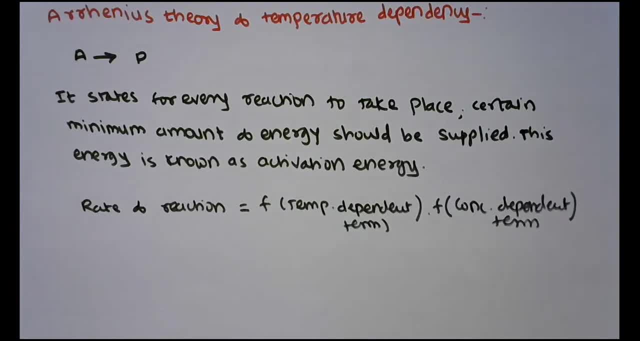 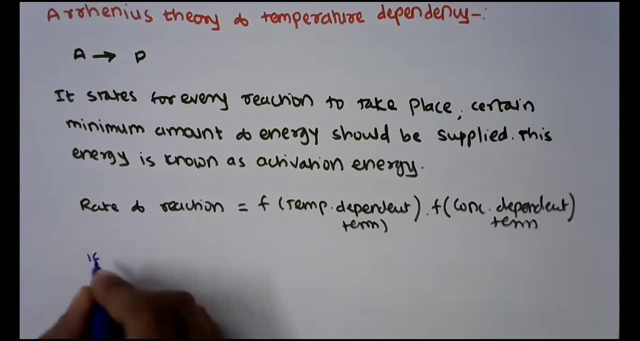 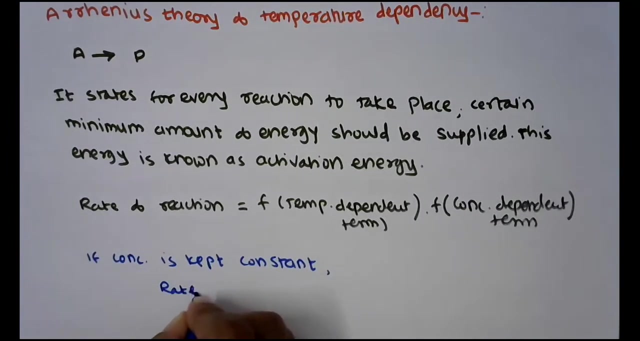 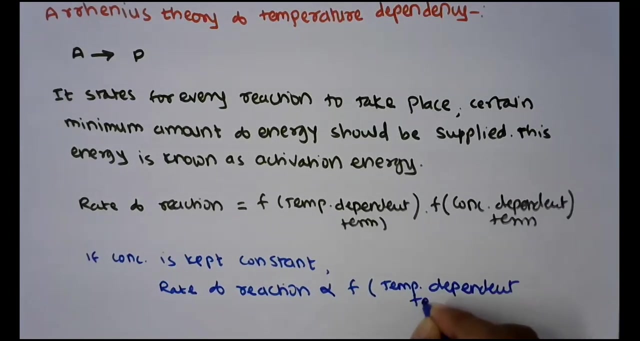 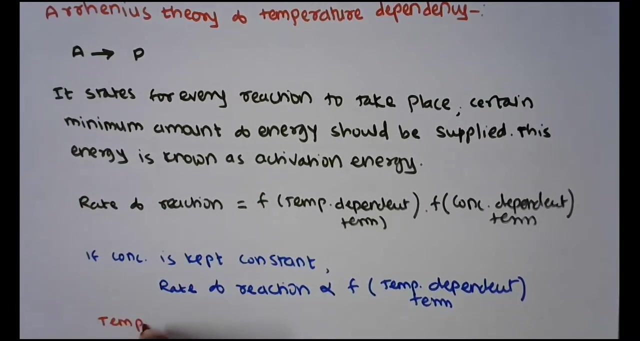 dependent term. Now, if we keep this constant constant, So if concentration is kept constant, then rate of reaction will be proportional to the temperature. So the rate of reaction is proportional to the function of temperature dependent term. Now, this temperature dependent term, the rate of reaction will be proportional to the. 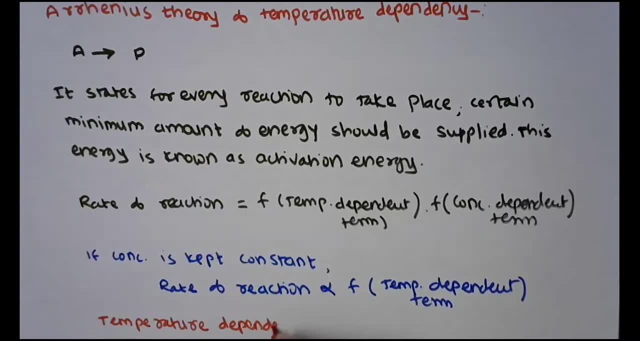 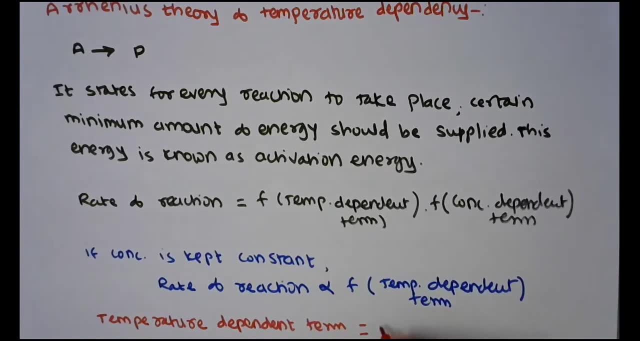 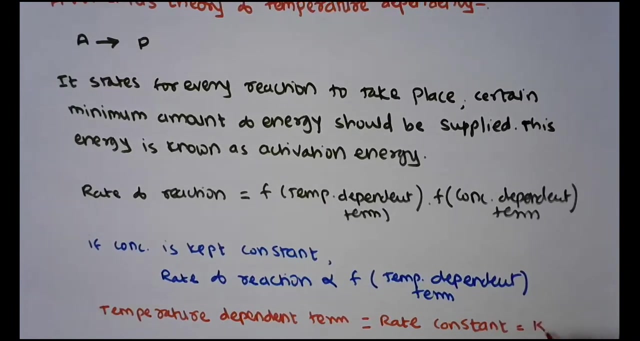 temperature dependent term. So it is equal to let us call it a constant, constant rate. constant Now, conditions will depend on the temperature dependent term. So in case we have a gas fit, in case the gas is completely nonpermanent, this temperature 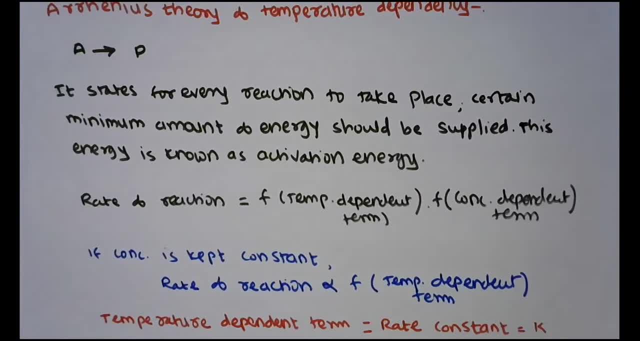 dependency, including Arrhenius theory of temperature dependency, correlate how the rate of reaction is affected because of the temperature. So now we will try to derive, or we will try to write the mathematical expression, we will simplify it, for the variation in temperature so as to understand the effect of temperature on the rate of reaction. 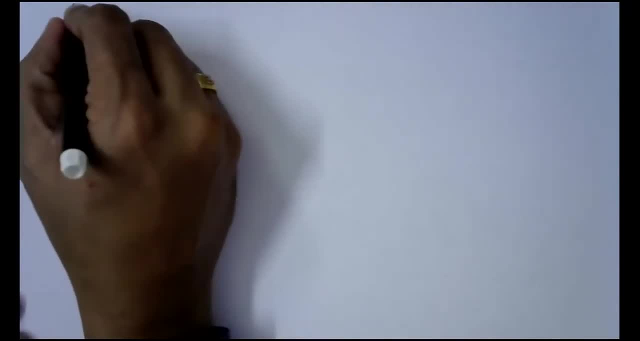 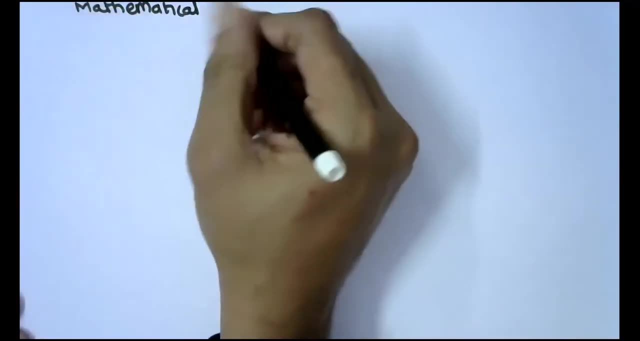 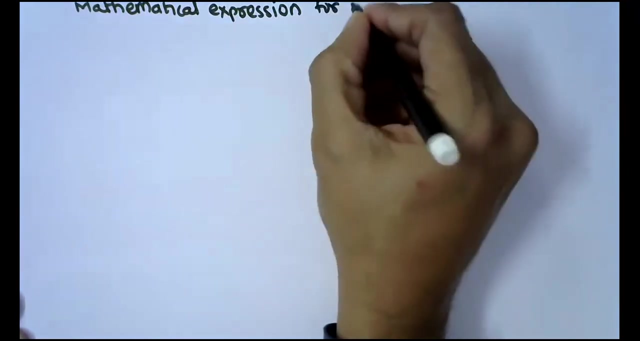 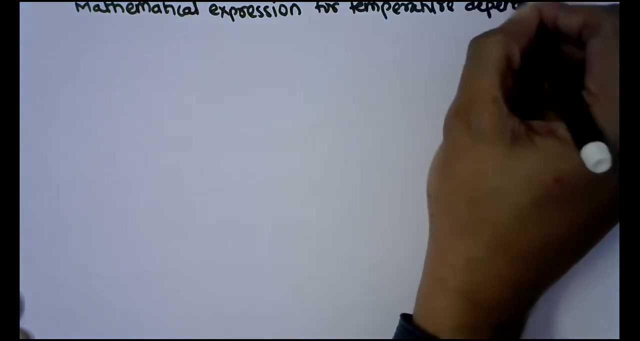 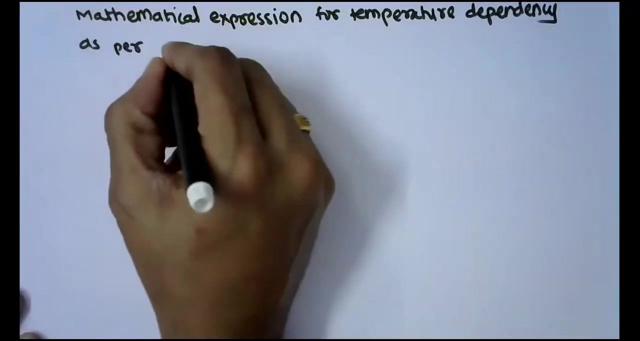 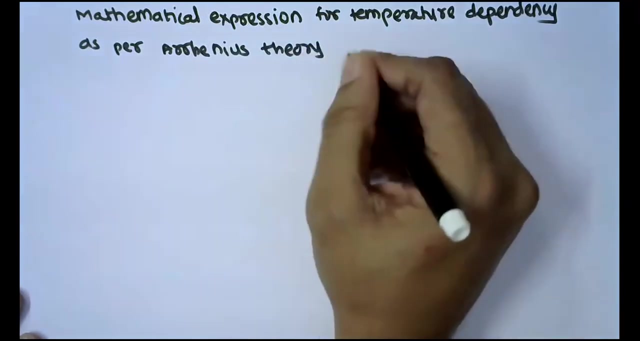 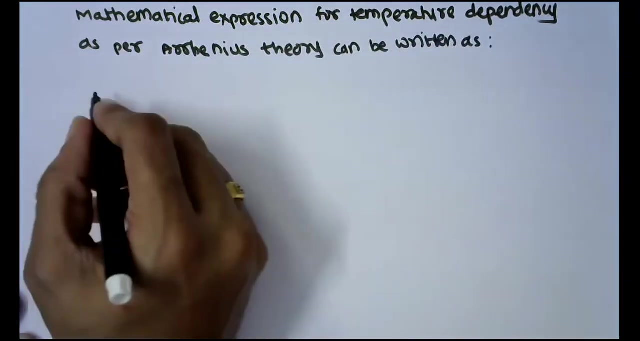 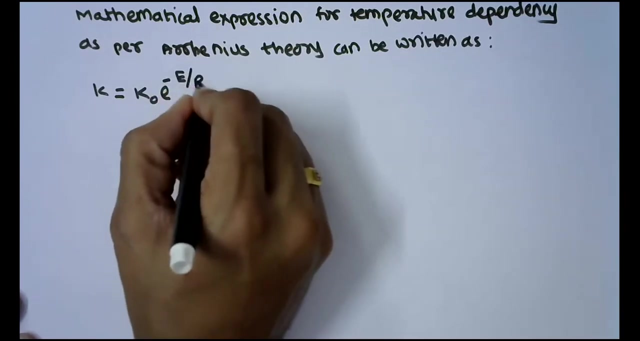 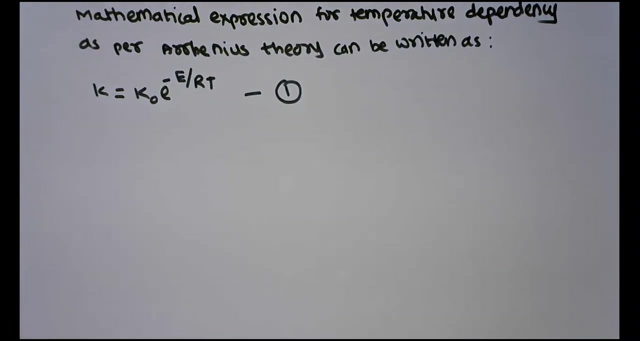 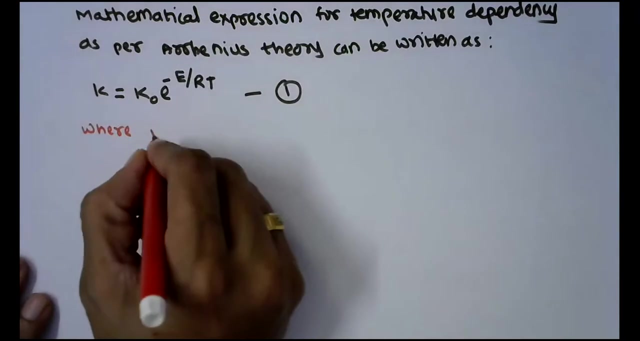 Now mathematically, or the mathematical expression for temperature, of temperature dependency, that is, per Arrhenius theory, can be written as: k is equal to k 0, e raise to minus e upon r t. this is equation number 1.. Now where? 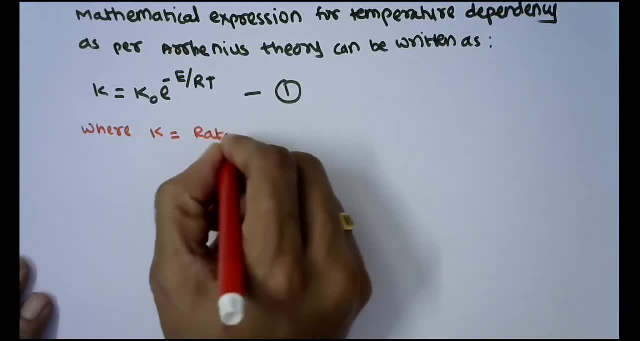 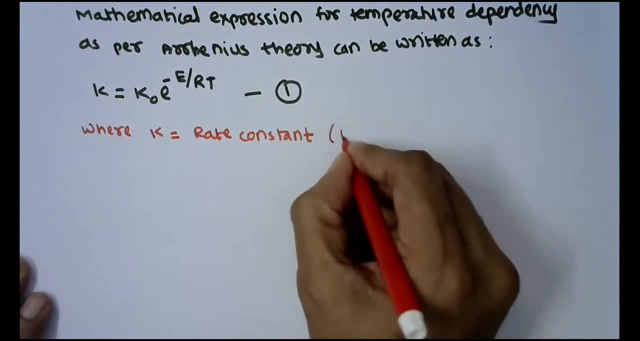 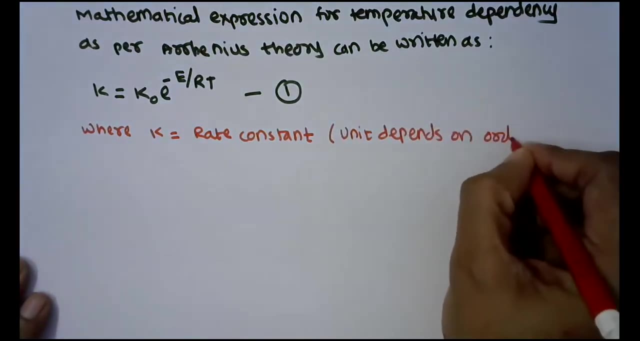 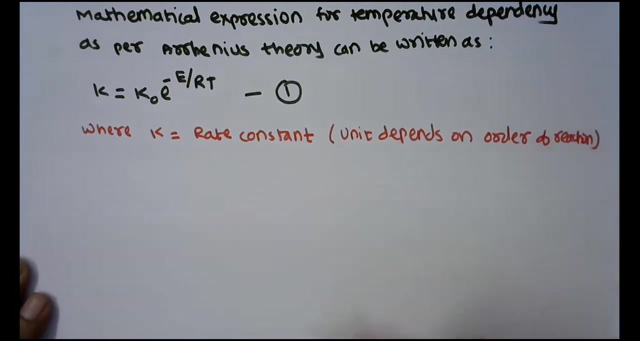 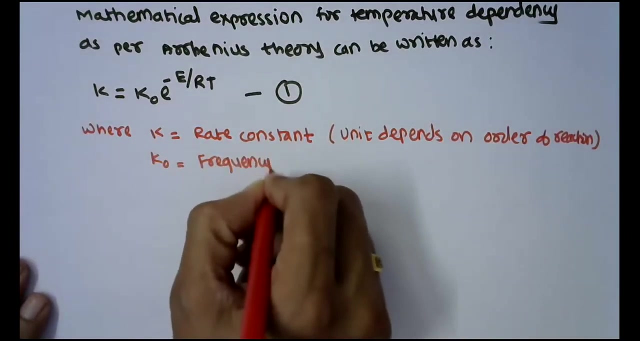 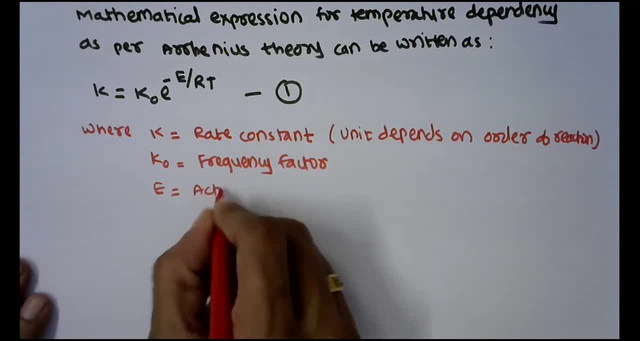 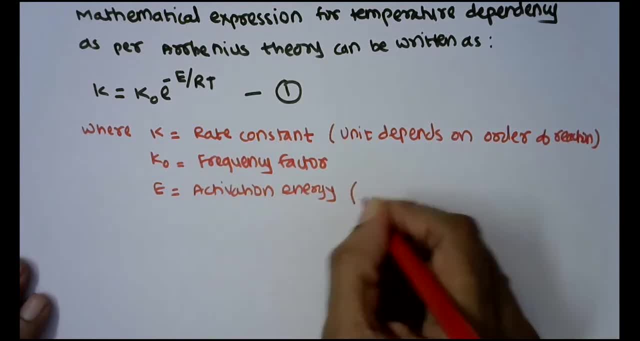 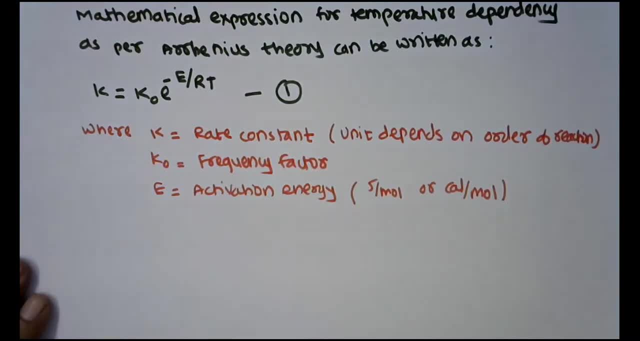 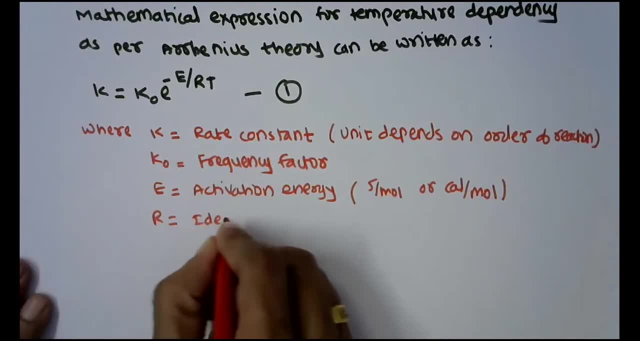 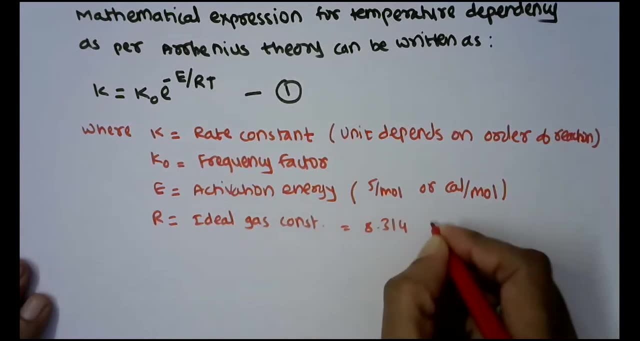 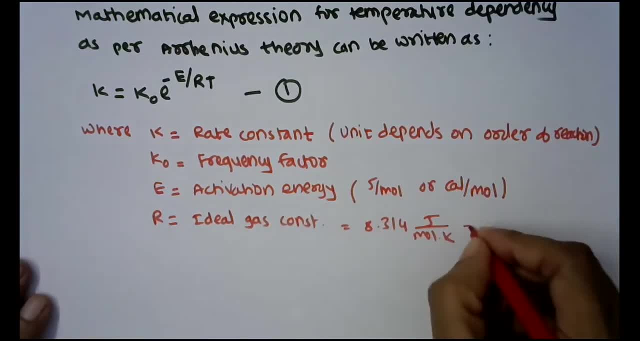 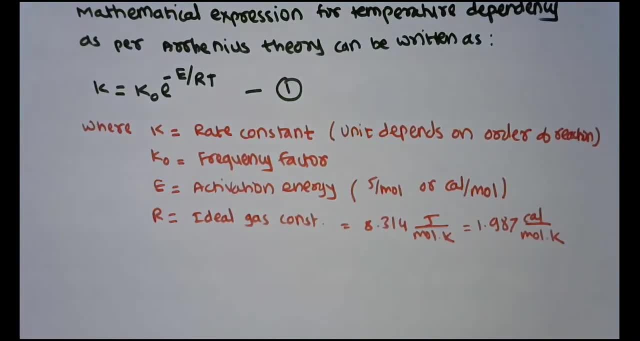 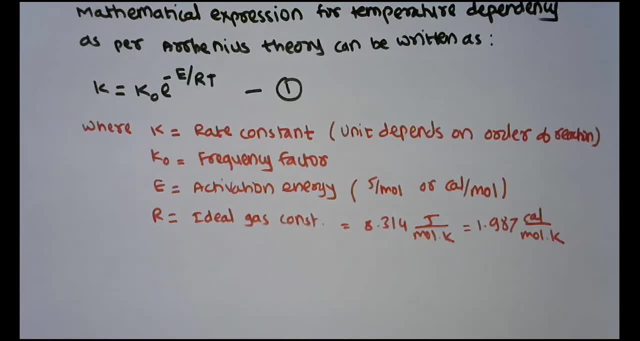 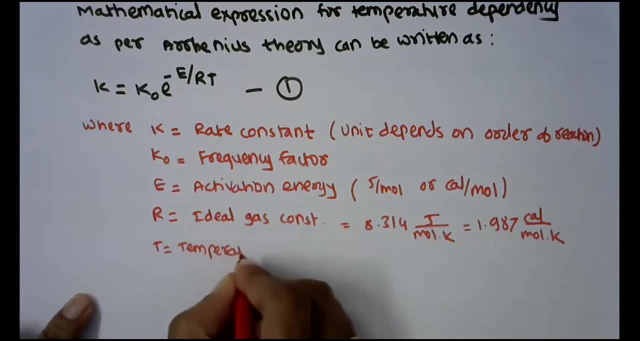 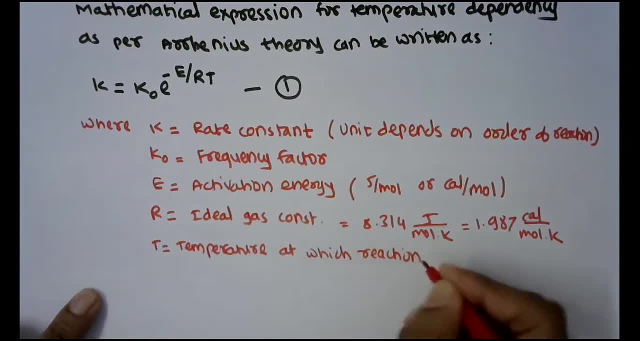 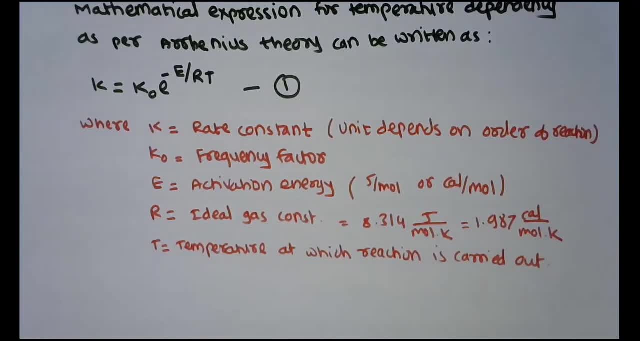 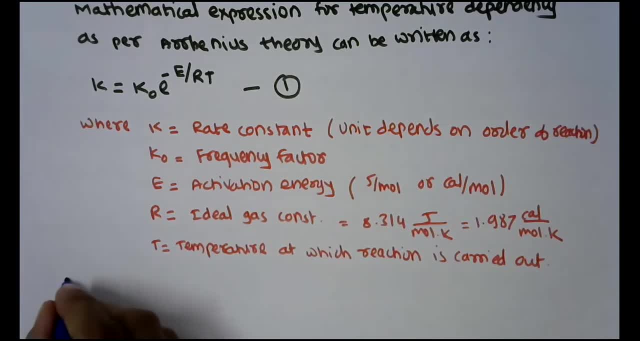 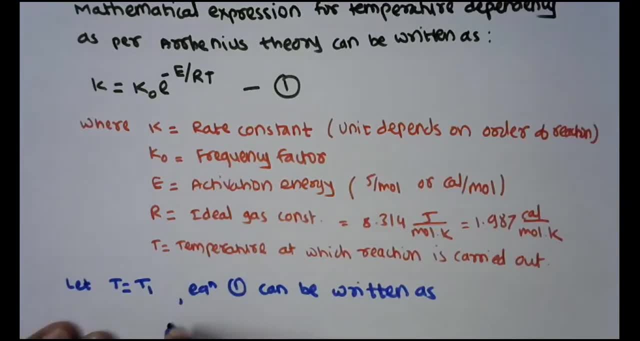 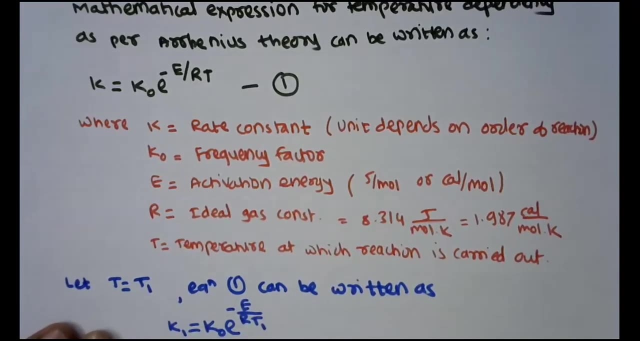 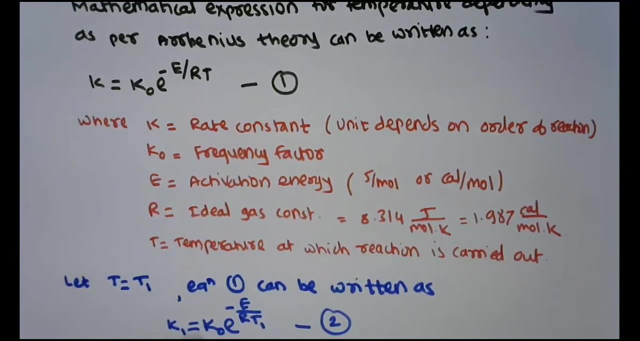 3, 3 k. 3, 2 k1 is equal to k0, e raise to minus e upon R T1. This is equation number 2.. Now this k1 means rate constant if the reaction is carried out at temperature T1.. k0 is a frequency. 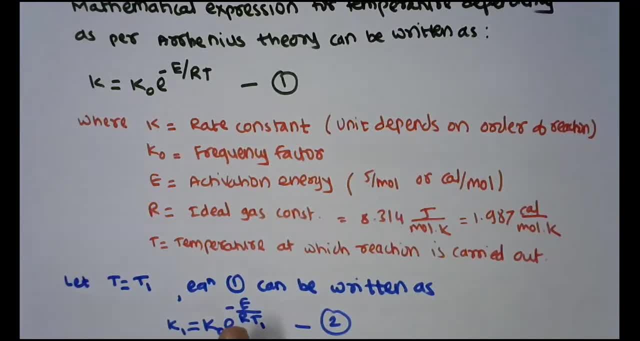 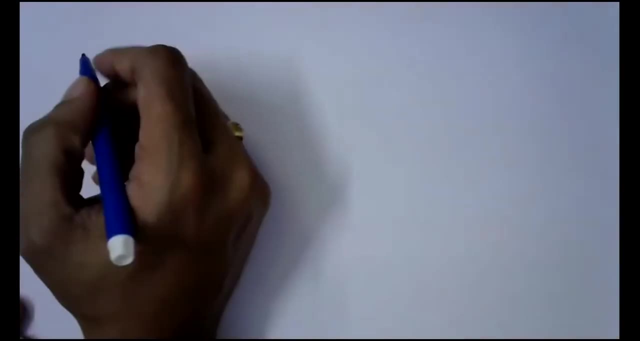 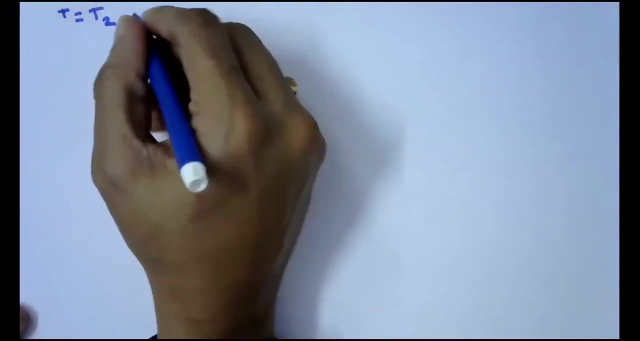 factor. It has the same unit as that of the rate constant. E is the activation energy, R is constant, R is ideal gas constant and T is equal to temperature T1 at which the reaction is carried out. Now consider another temperature: T is equal to T0.. So corresponding. 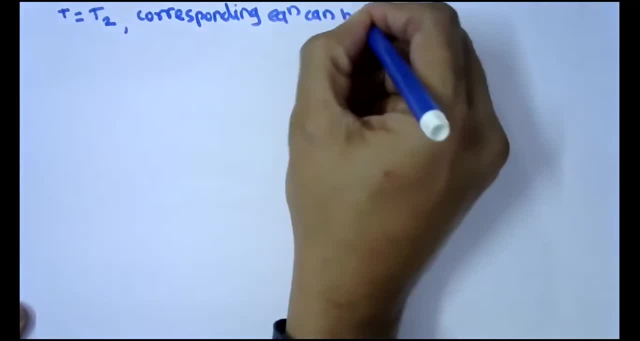 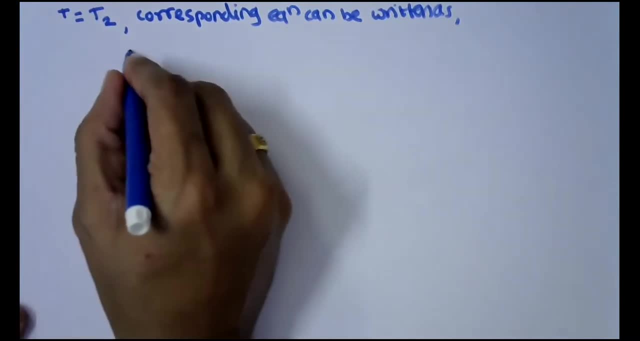 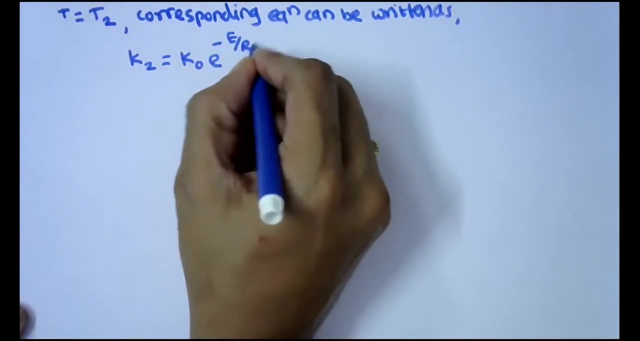 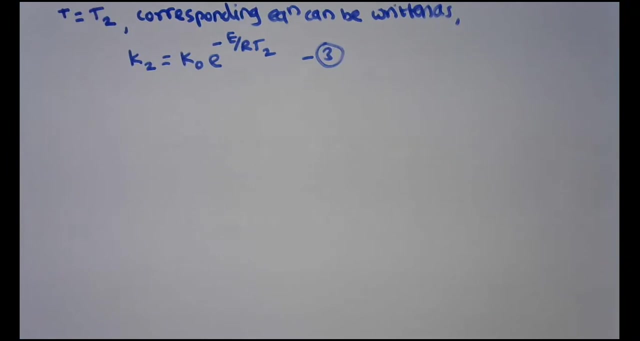 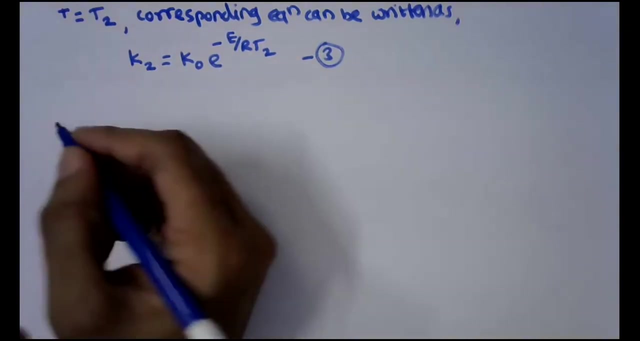 equation can be written as can be written, as: k2 is equal to k0, e raise to minus e upon R T2.. So this is equation number 2.. Now, in order to understand this equation, to what extent the reaction is accelerated, we have to divide equation 3 by equation to: 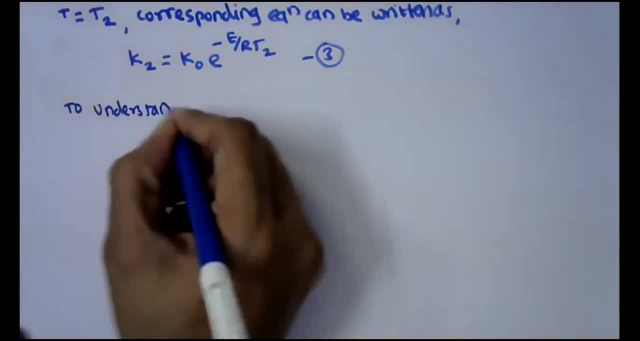 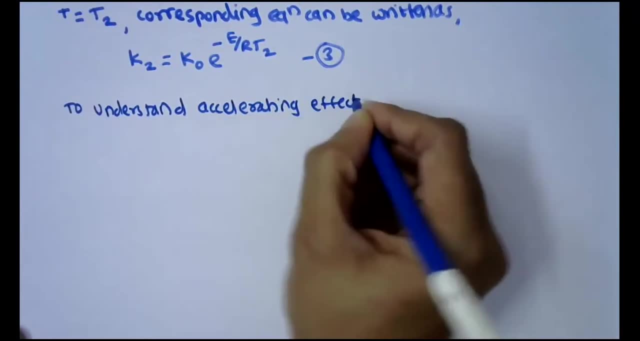 understand accelerating effect, effect due to change in the reaction momentum. So we should understand the value of x1 by y1, e raise to e as k1 by R, T1.. So now let us try this. So this is the equation number 2: k1 is equal to e, raise to minus e upon R. 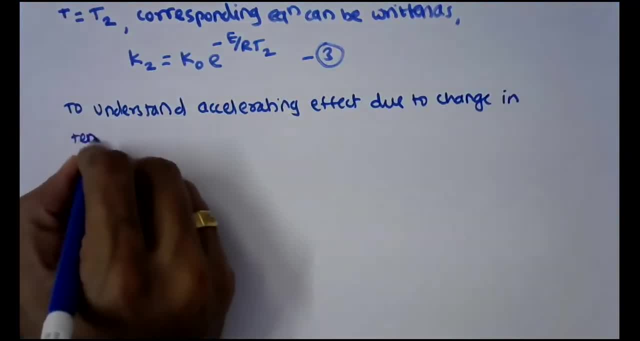 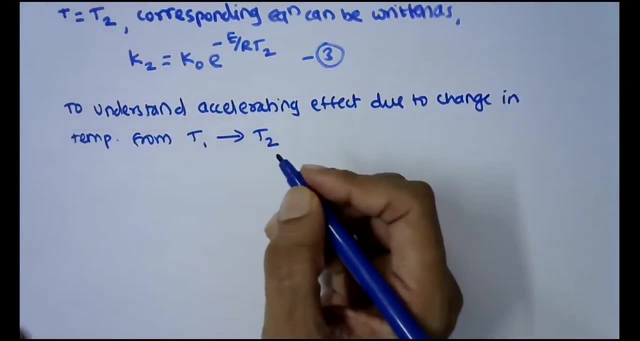 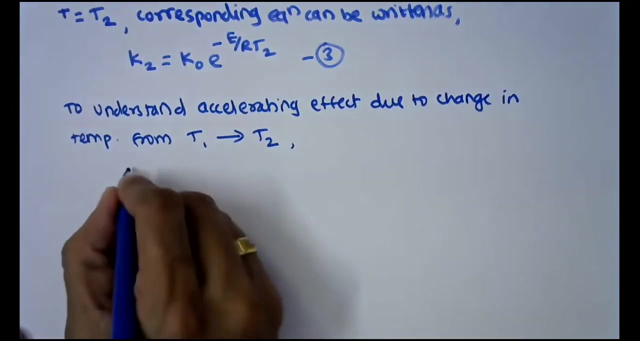 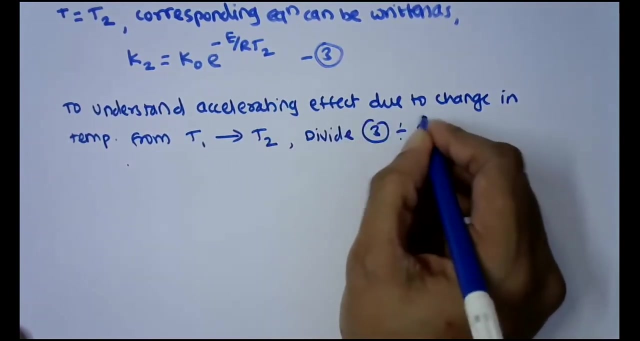 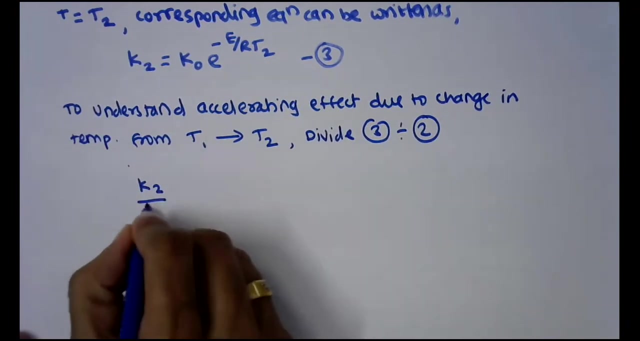 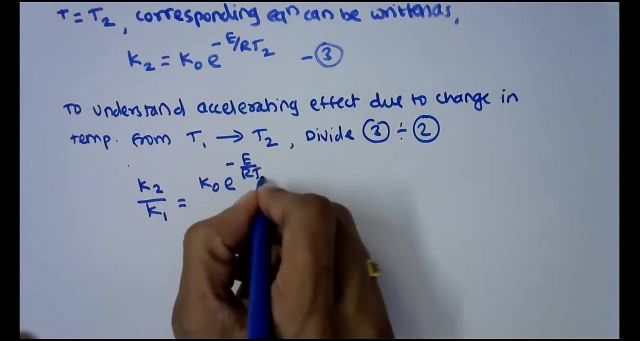 in temperature from T1 to T2, divide by 2.. So if we do 3 by 2, then what we get is: k2 upon k1 is equal to k0. e raise to minus. e divided by RT2, k0 e raise to minus. 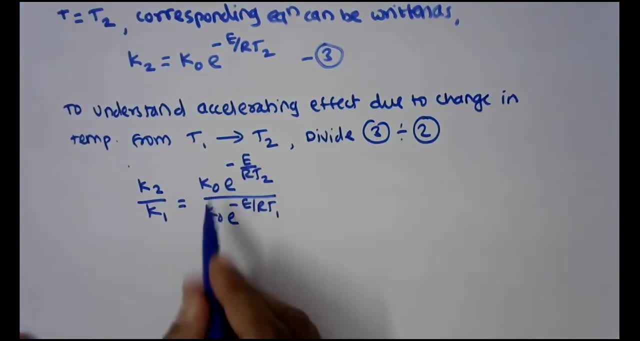 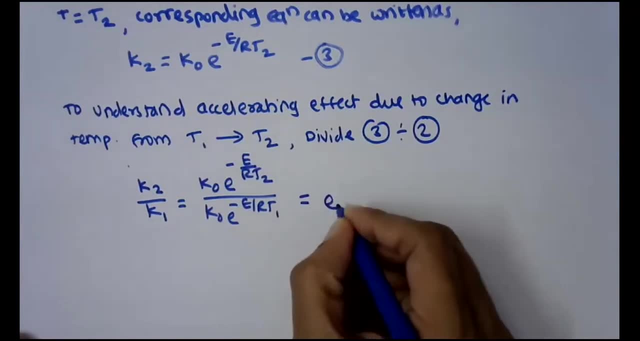 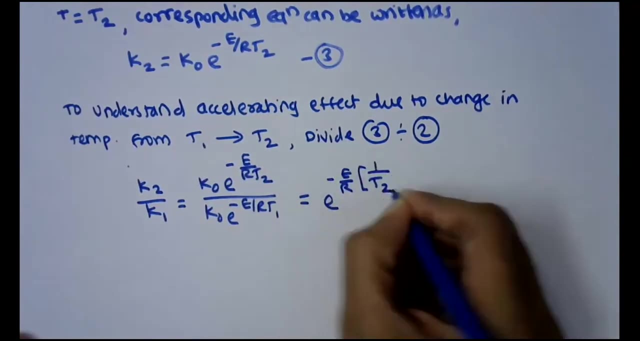 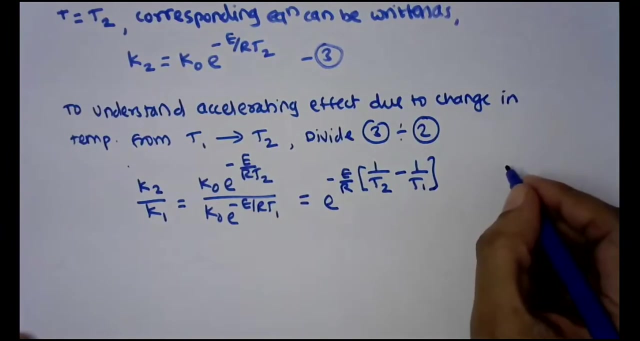 e upon RT1.. So this k0 k0 will get cancelled and we may simplify it as e raise to minus e upon R, inside the bracket 1 by T2, minus 1 upon Tn. Now here the formula which I have: 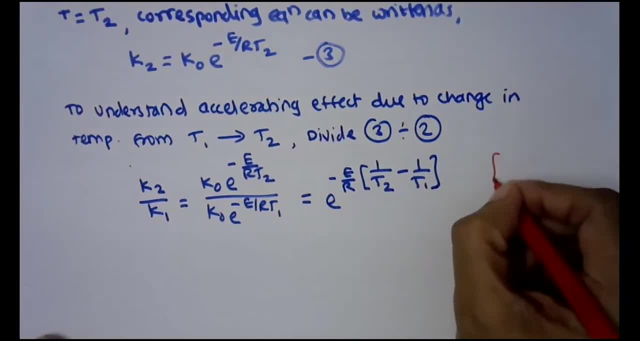 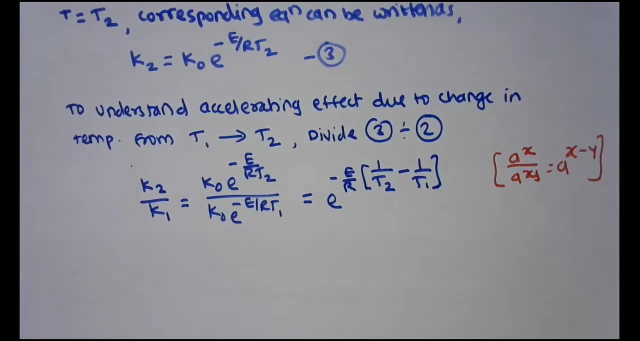 considered for simplification is the law of indices: a raise to x upon a raise to y is equal to a raise to x by y. So now let this is equation 4, or we will rewrite again. k2 upon k1 is equal to e raise to minus. 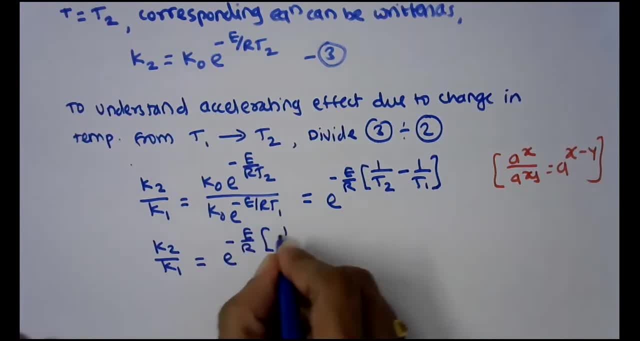 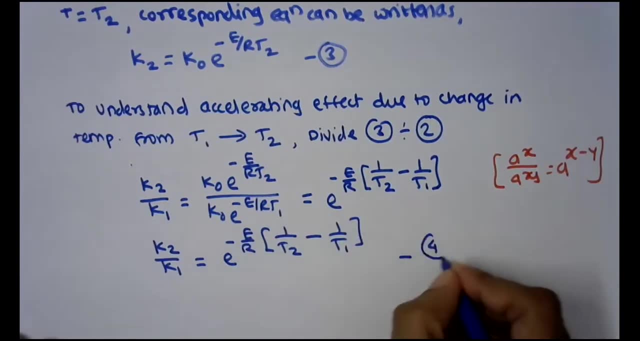 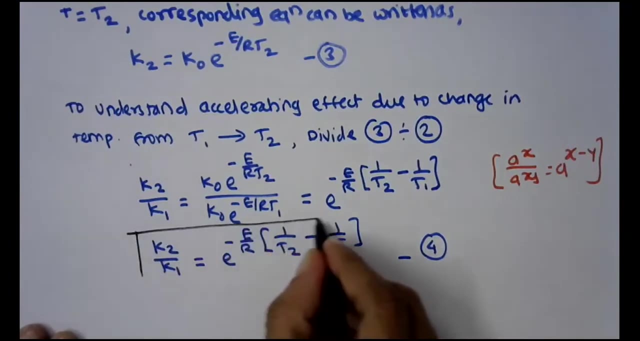 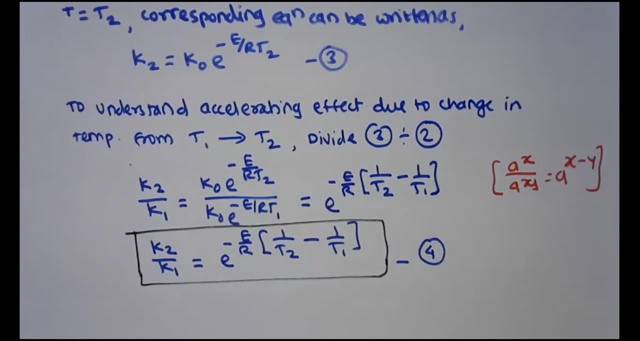 e upon R into 1 by T2 minus 1 upon k1.. This is equation 4.. If we substitute the value of R- activation, energy and two temperature, then it will give us an idea about how much the rate will be accelerated if the same reaction at same condition. 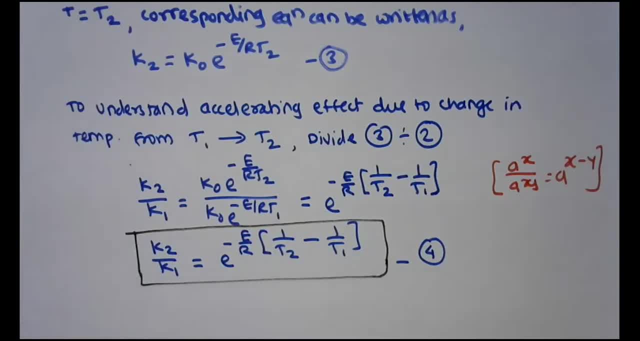 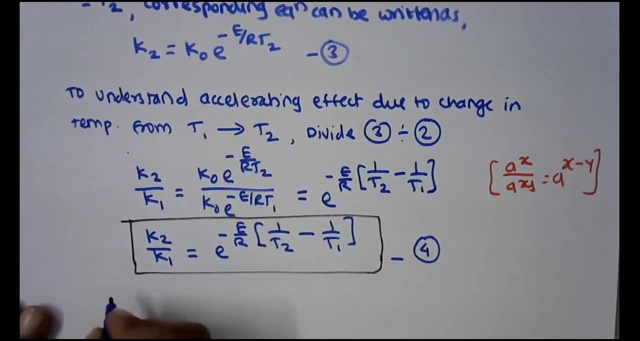 is carried out at two different temperature: T1 and T2.. Now this can be further simplified by taking the log. Now take ln of equation 4.. Now, if we take ln of equation 4, then we can get l of. 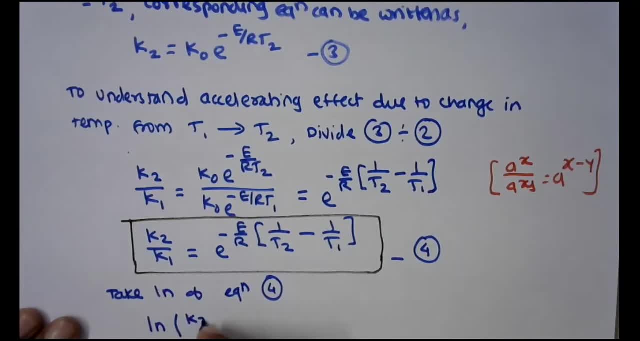 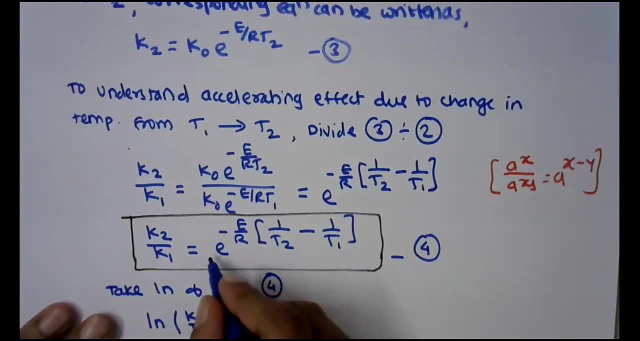 Ok, So kidding. So we did not do So, So we did not, So we did not. k2 divided by k1 is equal to now. it will be ln of e raised to minus e by r into 1 upon t2 minus. 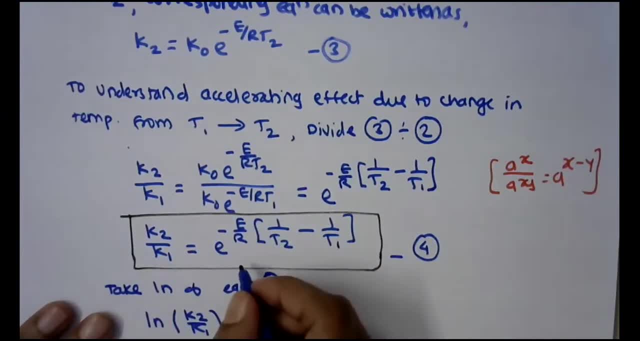 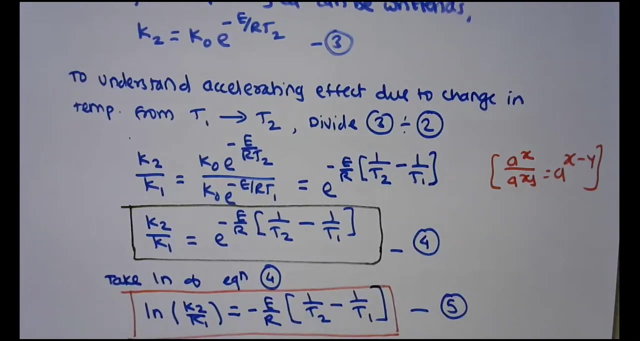 1 upon t1.. So ln of e to the base is 1, so I can directly write as e upon r inside the bracket bracket. This is equation number 5.. So this is a simplified form of the mathematical expression of Arrhenius law. So this is another form. Now you must be able to remember that. 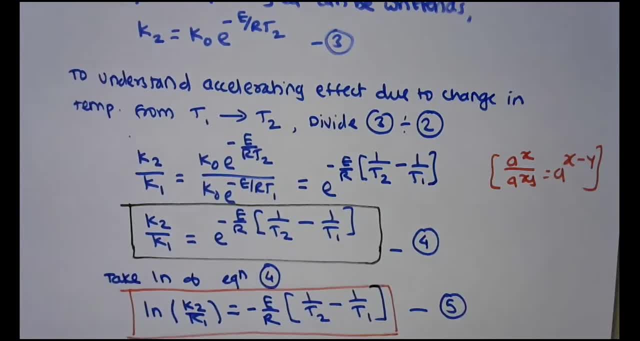 I said that this is the equation number 5.. So this is the equation number 5.. So this: I said that the rate of reaction is accelerated if the same reaction is carried out at a two different temperature. It is said that for every 10 degree rise in temperature, the rate 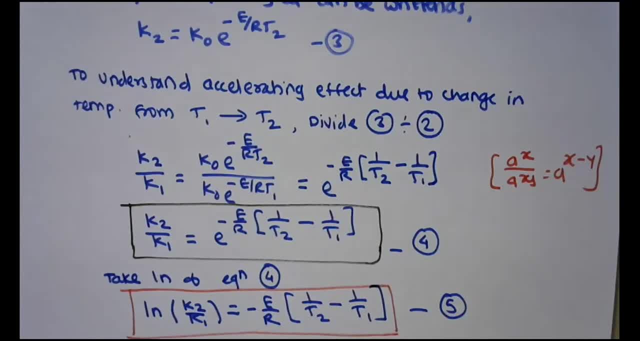 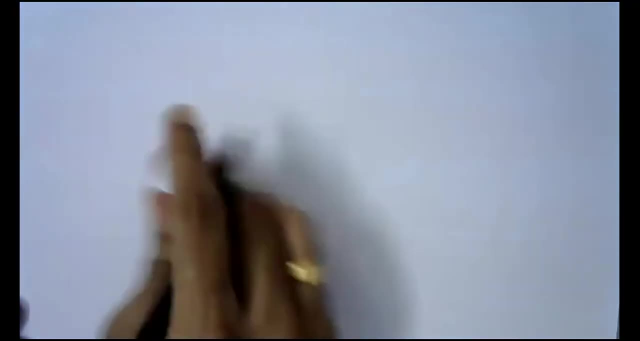 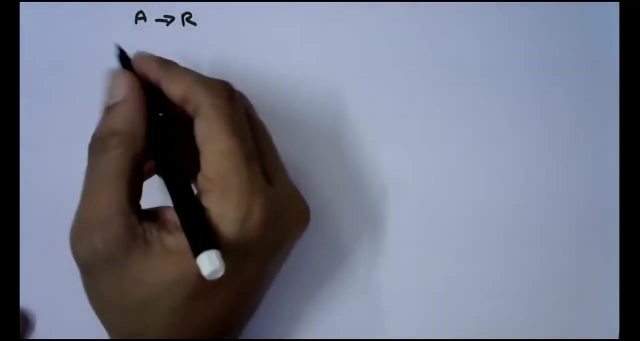 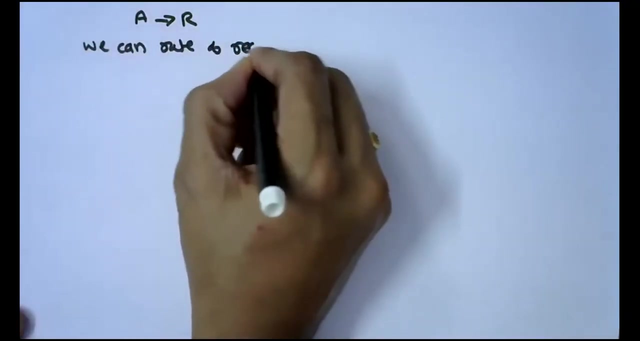 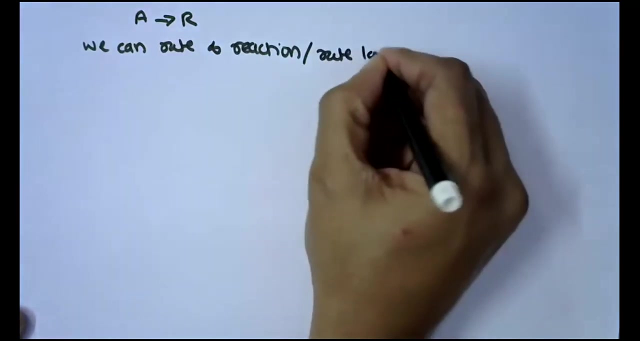 of reaction doubles. Now we will try to rewrite this equation 5 in terms of rate of reaction. So, considering reaction A gives R, considering the reaction A gives R, we can write. we can write rate of reaction, or rather rate law expression. 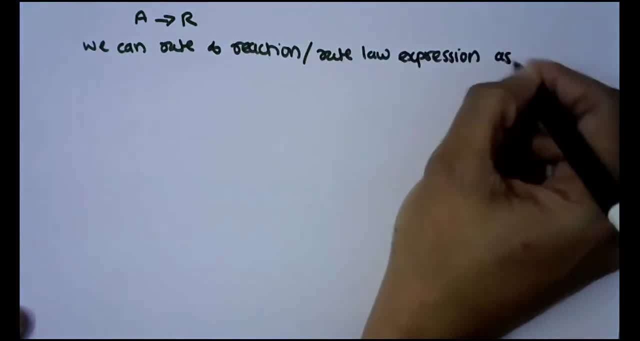 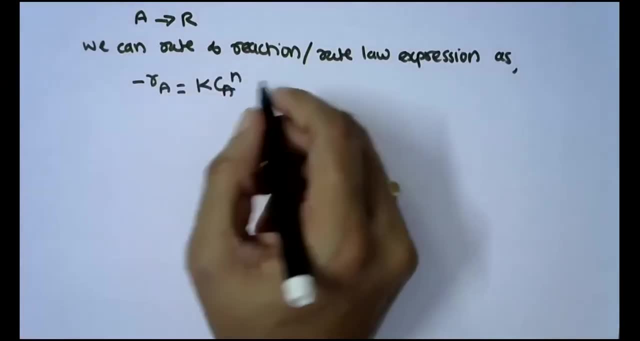 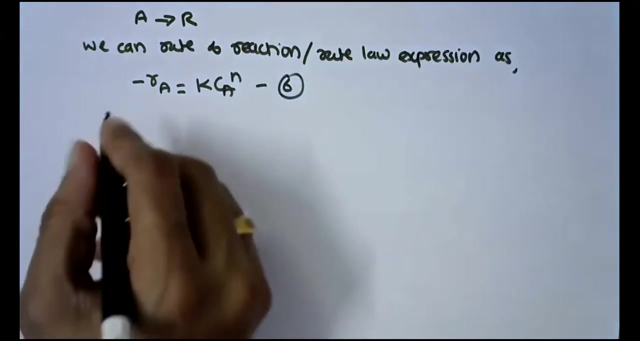 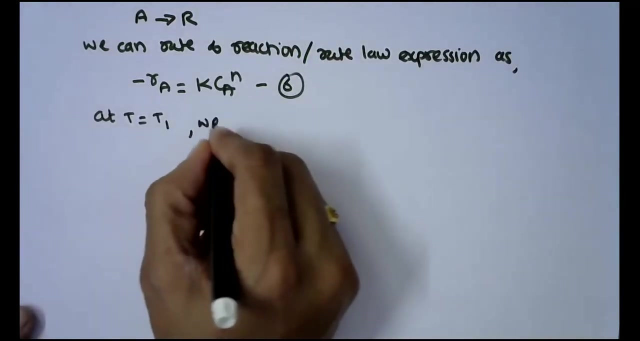 Let us consider it as S minus RA is equal to kcA. raise to mz. So consider this as equation 6.. Now had T is equal to T1, we can write: we can write that at t is equal to t1, we. 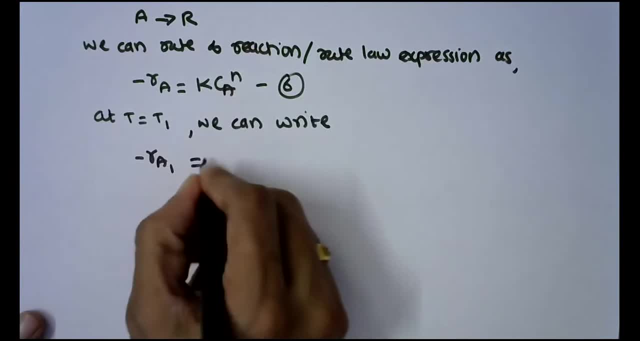 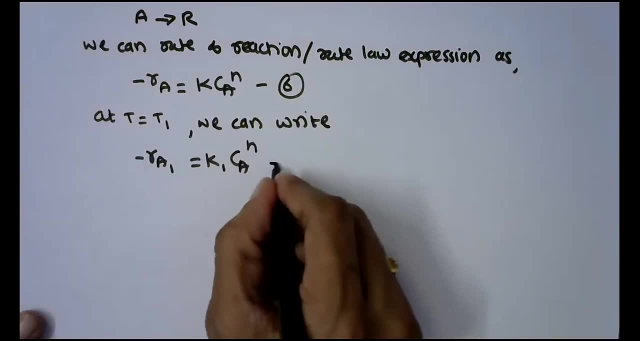 can write that. So we can write: T is equal to t2,, S is equal to p1.. So this is the distribution. Red film chloride minus Ra1 is equal to k1. Ca. raise to n. Now say: this is equation 7.. Now you. 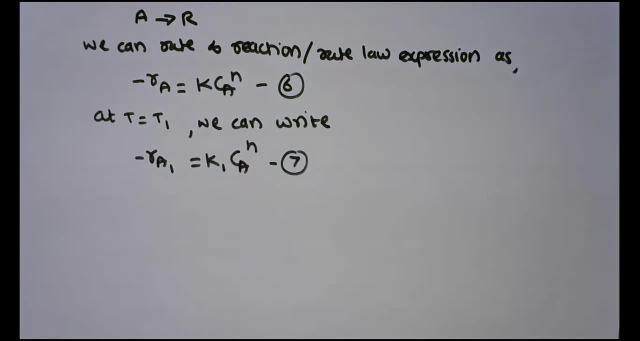 may say that, sir, why we have not changed the concentration. The reason is we are not studying the effect of concentration. We are studying the effect of temperature, The reaction mixture of the same composition. we are just trying to carry out the reaction at two different 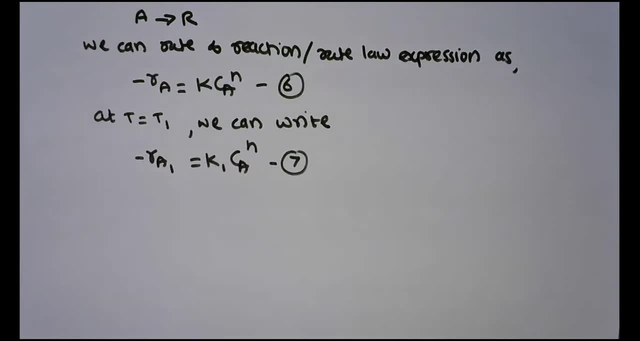 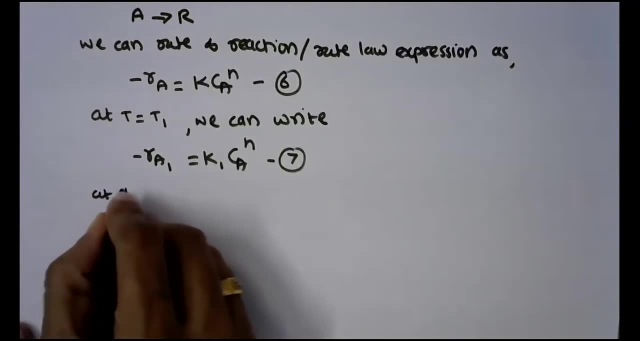 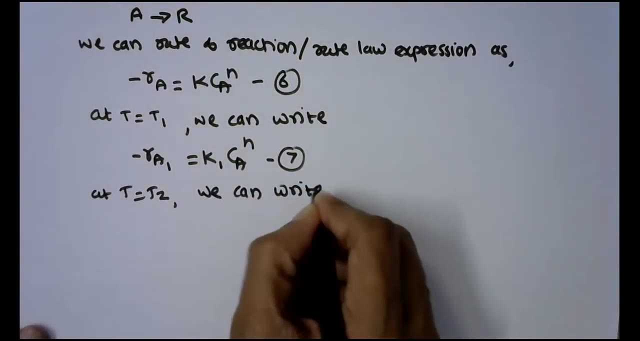 temperature at same operating conditions, including concentration, just to understand the effect of temperature. So similarly, at T is equal to T2, we can write: minus Ra2 is equal to T2.. So we can write: minus Ra2 is equal to T2.. So we can write: minus Ra2 is equal to. 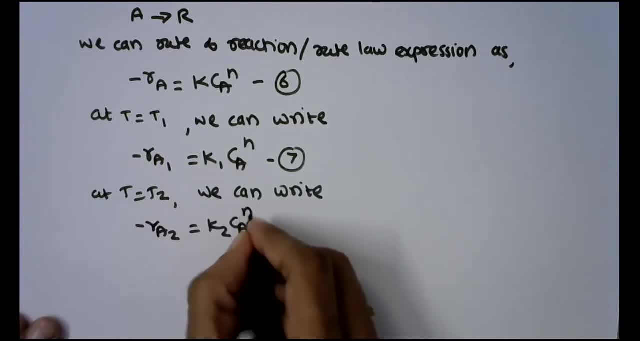 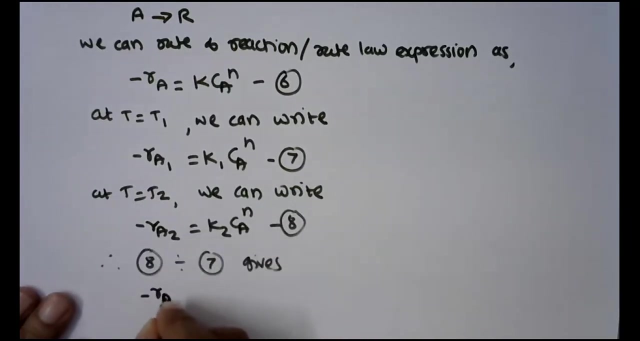 K2 Ca raise to n. This is equation 8.. Therefore, 8 divided by 7 gives. now please try to understand minus Ra2 divided by minus Ra1.. K2 Ca raise to n divided by k1 Ca raise to n, So Ca raise to n, Ca raise to n will get. 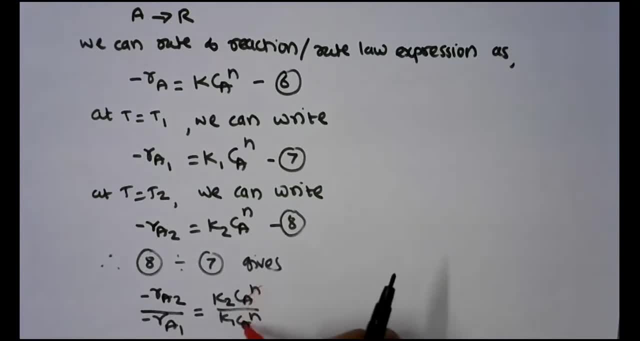 cancelled. This Ca raise to n, this Ca raise to n will get cancelled and therefore this minus Ra2, this minus Ra2 by minus Ra1.. The first thing that is needed to be Powertrain equation: Ca raise to n will be equal to Ca. 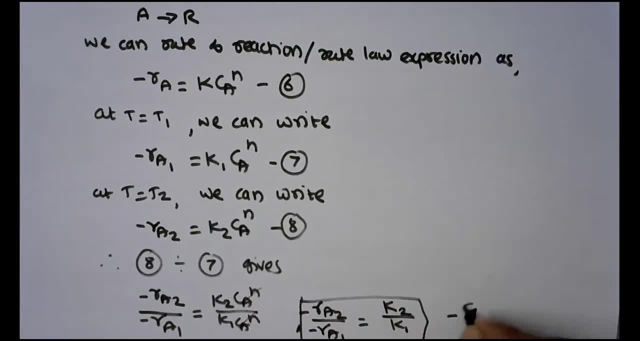 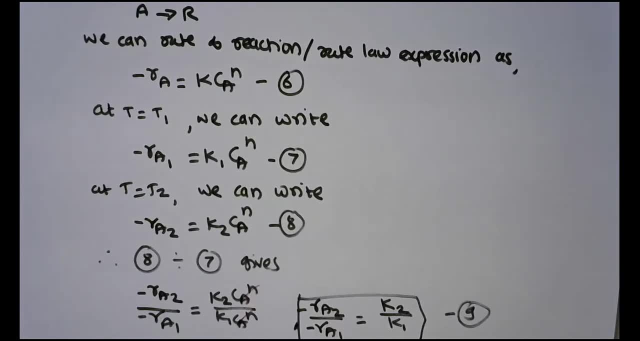 raise to n greater than Ca, raise to n by 4 or bigger than 4 by r. e to verde working. what we can do is we can replace K2 by K1, either in equation 4 or equation 5, by minus Ra2 by minus 5.. So that is by 6.4, we come here. this is equal to 0 by 1 by k1.. Now make: 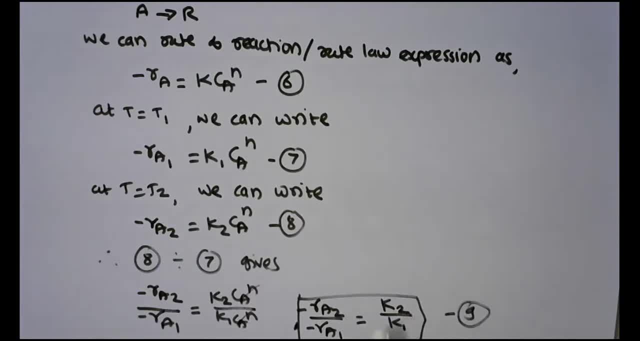 RA1 or the ratio by which even this itself can prove that the ratio by which the rate constant is exchanged by the same ratio, the rate of reaction will also change. So if rate of reaction doubles for every 10 degree Celsius rise in temperature, it means the value of rate constant will also. 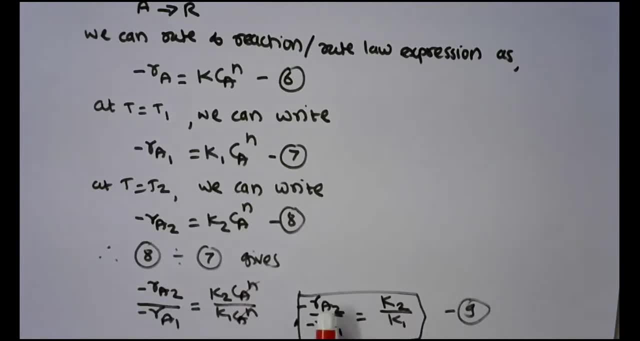 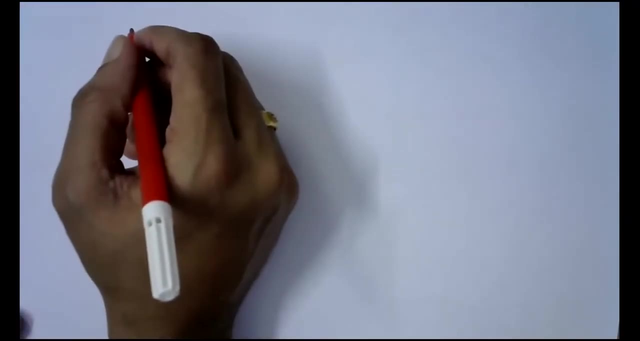 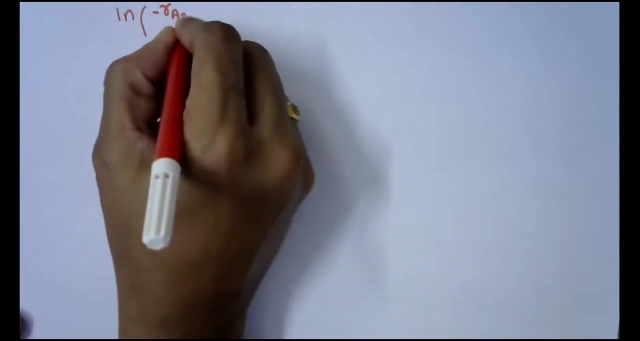 double. So just for the sake of understanding, replace k2 by k1 by minus RA2, by minus RA1 in equation number 5 and rewrite the equation. So let us write ln of now. I am writing in place of k2 by k1, the terms of rate is equal to: 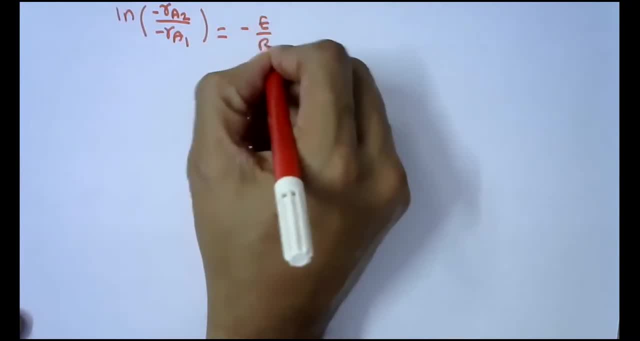 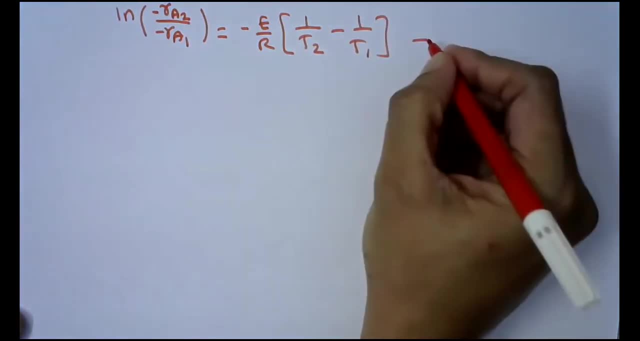 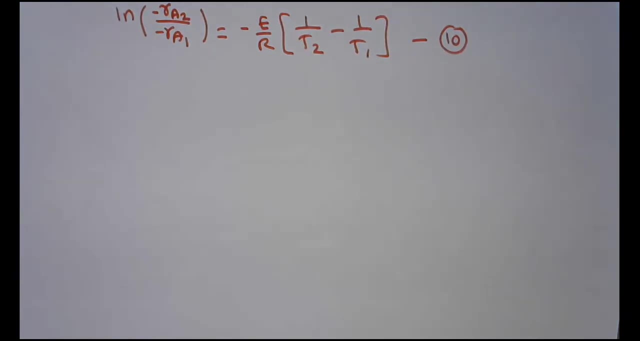 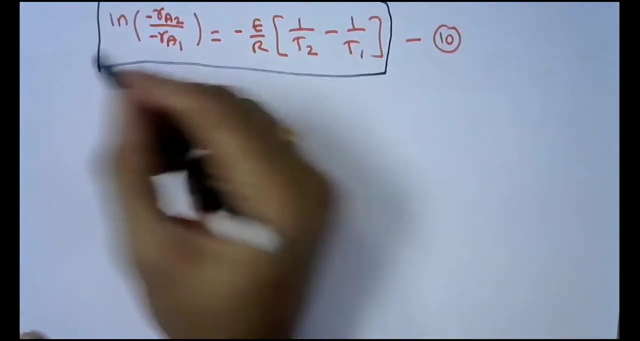 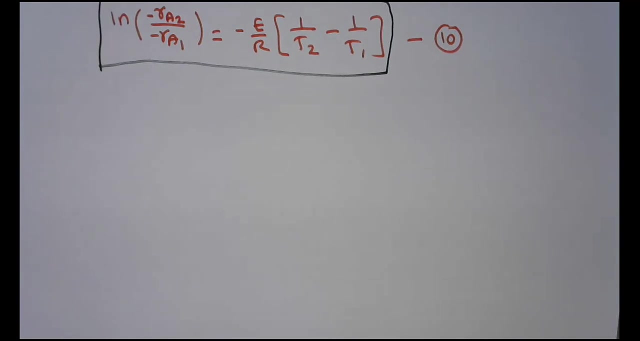 R or minus E upon R, inside the bracket 1 upon T2, minus 1 upon V1. equation Q: completely X. So in this way we have tried to understand, we have tried to understand the accelerating effect of the temperature on the value of rate constant and thereby on the rate of reaction. Now this: 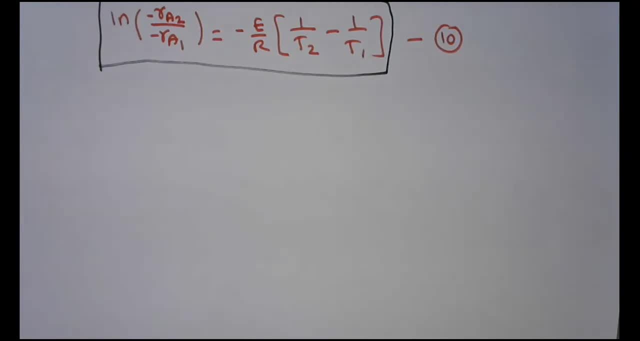 situation can be understood either by solving the problems by substituting the condition of temperature and R and activation energy. but we can solve this graphically also, And you must have realized by this time that if the value of K2 by K1 and T2 and T1 and R is given, 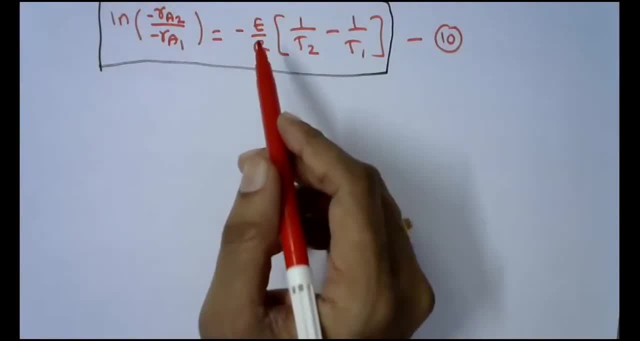 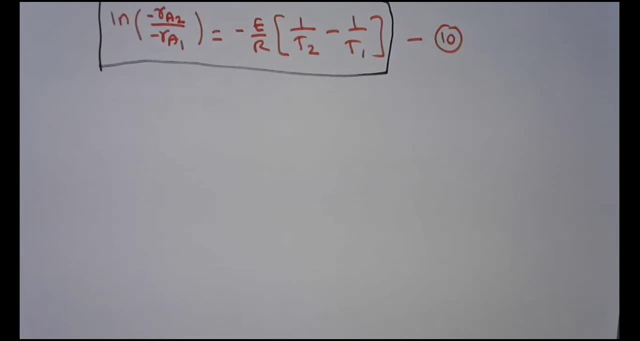 we can find out activation energy, or if activation energy, R and 2 temperature is given, you can find out the ratio of K2 by K1 or minus RA2 by minus RA1 or any unknown. Now let us consider again the equation 3, equation, rather the basic equation, So I will rewrite the same. 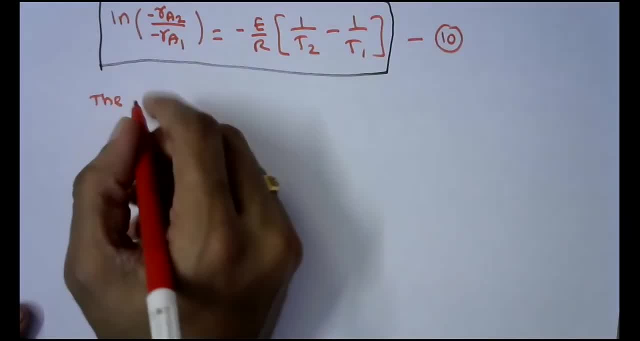 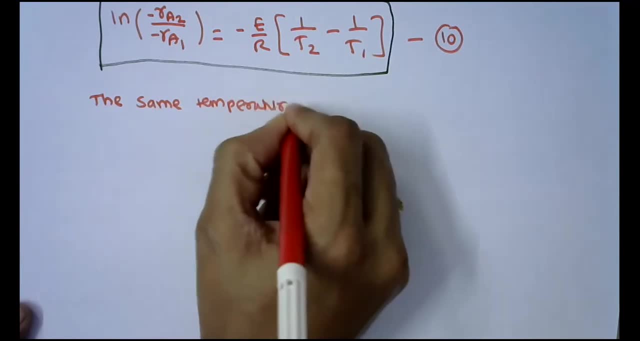 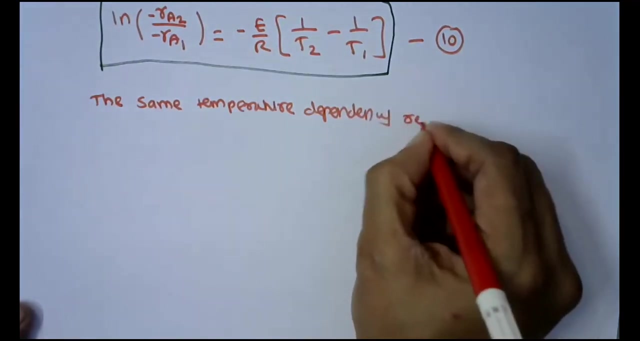 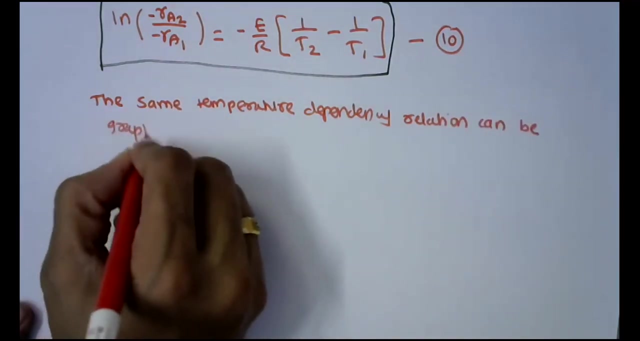 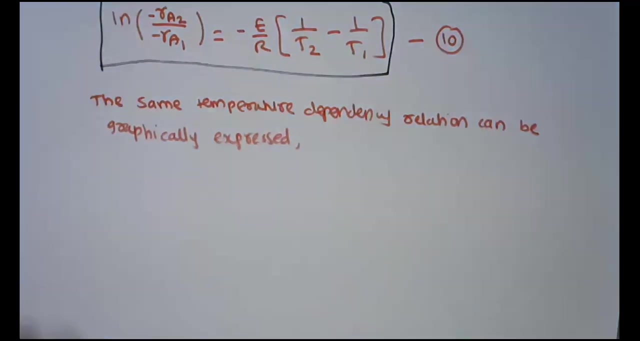 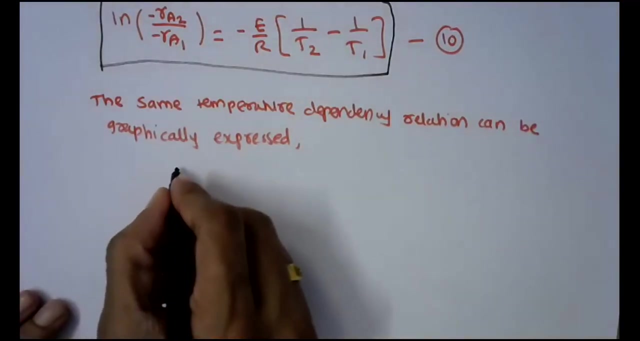 the same temperature dependency relation can be graphically expressed, Expressed, or rather, can be estimated graphically. Now, how will you do it or how will you estimate it graphically? So the mathematical equation of Arrhenius equation is: K is equal to K0, e raised. 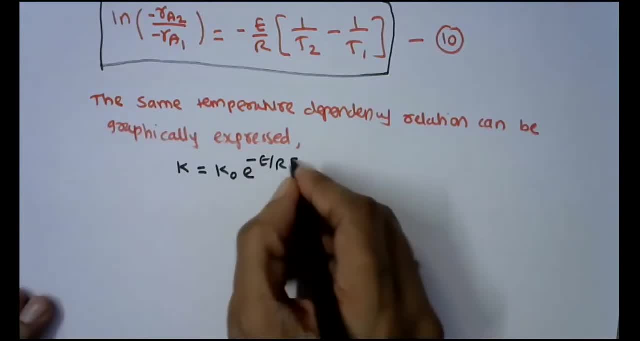 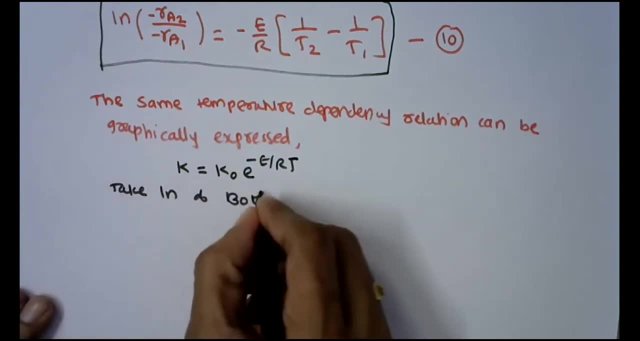 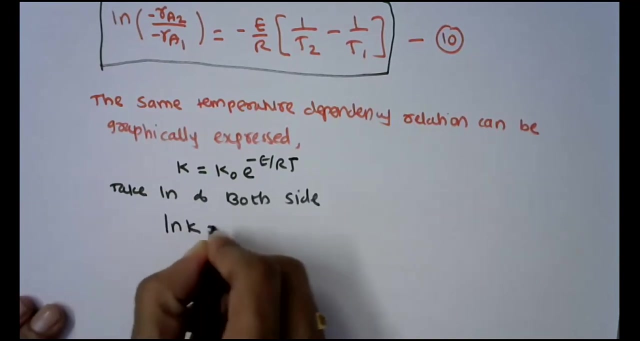 to minus e upon RT. Now take a look at the equation 3, equation rather the basic equation, So I will rewrite the same. you take a likeng of both sides. If you take an ln of both sides, then you will get: ln of K is equal to ln of K0. 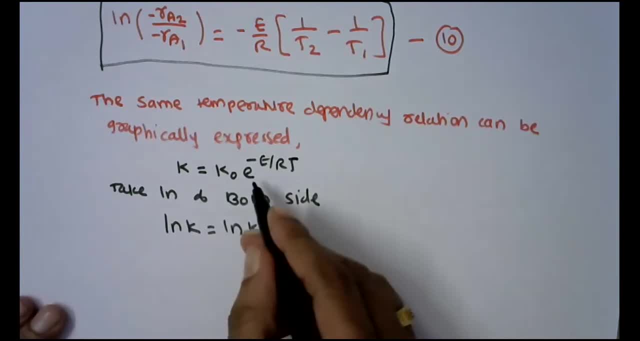 Now ln of now plus plus ln of e raised to k, e raised to minus e, bar RT. if you simplify, then it will be simply, And this is of the form: y is equal to c plus m, x and therefore, therefore, if you plot the, 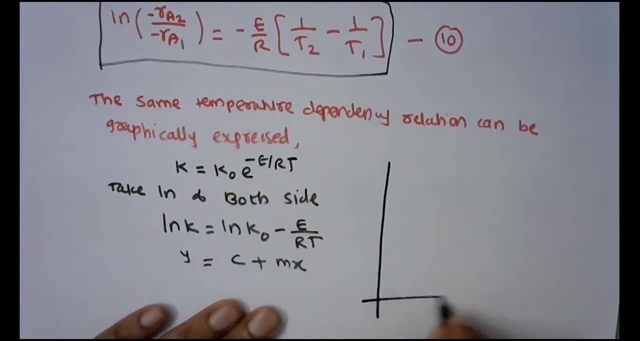 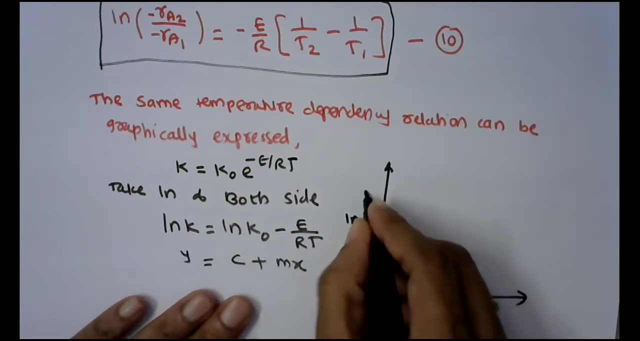 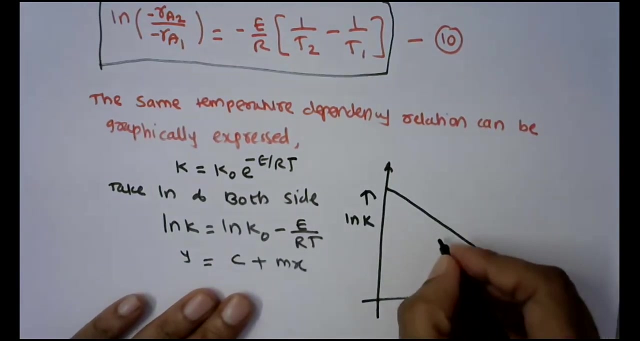 graph of. if you plot the graph of ln of k versus 1 upon t, then you will get the relationship like this: and the slope will be equal to minus t upon will be equal to minus e by r and the value of intercept will be equal to ln of. 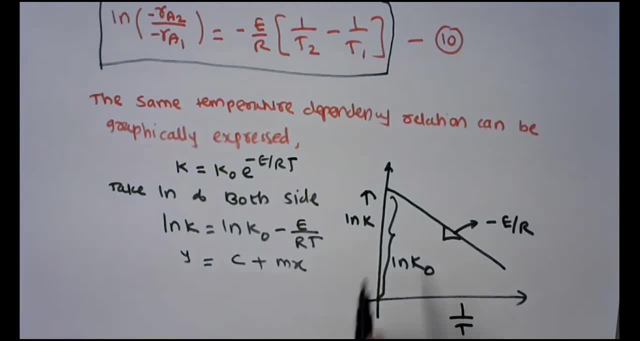 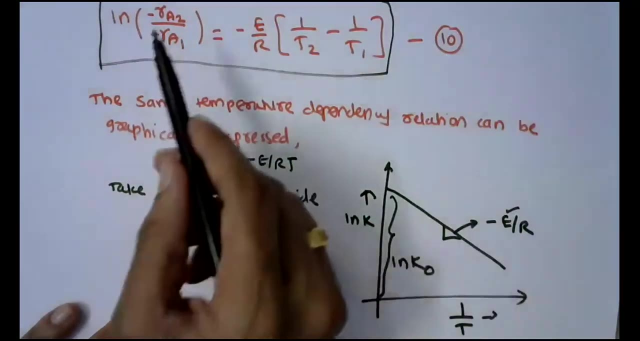 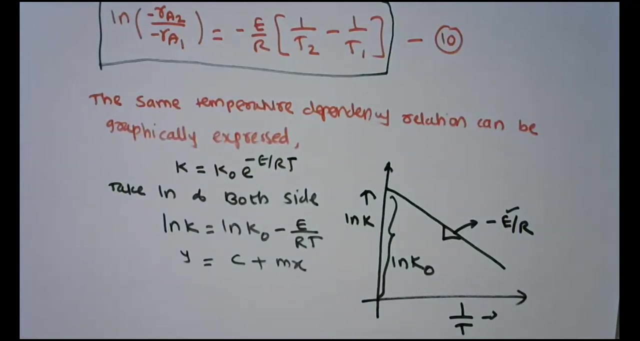 k 0.. So if the value of the rate constant at different temperatures are given, then by graphical method also you can determine the value of activation energy. or if just two values are given, Then you can substitute either in equation 5 or equation 10, depending upon whether the 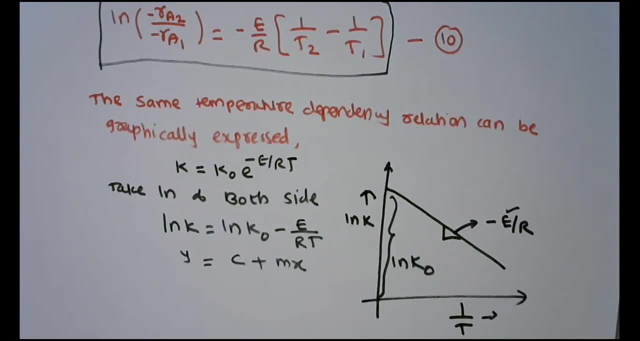 rate or rate constant is given and the problem can be solved. So in this way, using the Arrhenius theory of temperature dependency, the effect of temperature on the rate of reaction can be understood. Now the slope, this slope of the reaction energy is given and the slope of- I give the 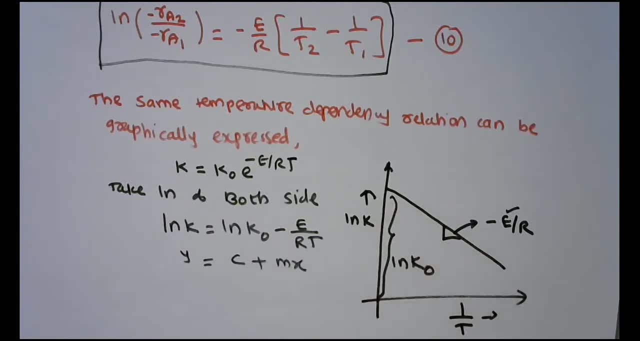 rate of reaction can be understood. So the slope of the rate of reaction can be calculated by the temperature of the reaction. of this ln of k versus 1 by T graph depend upon whether the reaction or depending upon the temperature at which the reaction is carried out, or depending upon the value of activation. 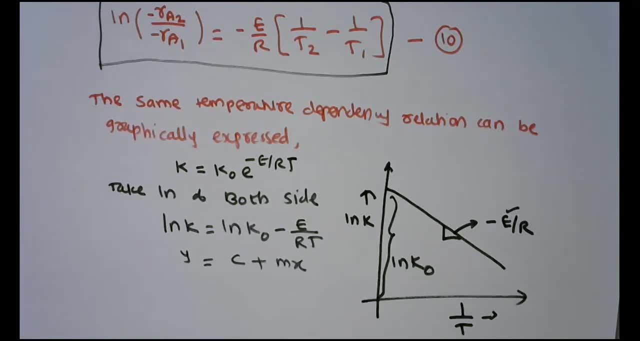 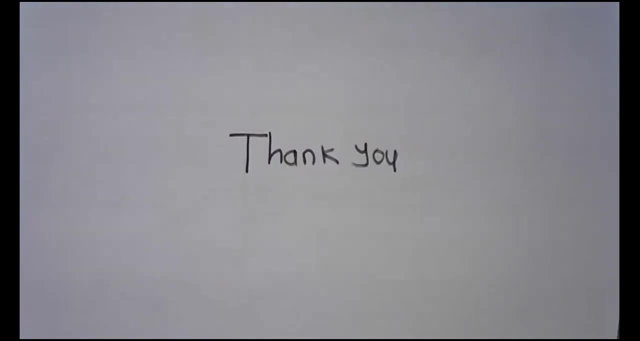 energy. So, depending upon the value of activation energy, the temperature sensitivity of the reaction will differ and accordingly the slope of this curve, of this straight line, will also differ. So thank you for watching this video and in this video, step-by-step, I have tried to explain how the temperature dependency of the rate constant using Arrhenius. 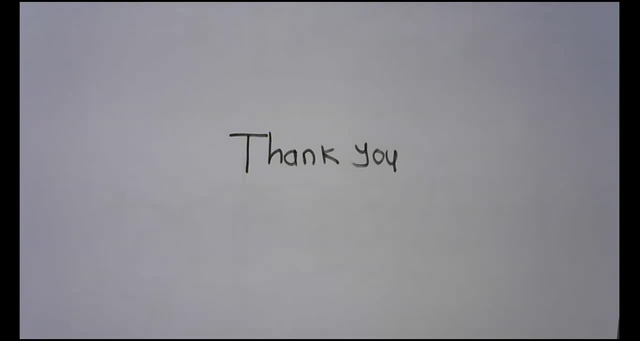 theory is expressed mathematically And how the reaction would get more accurate. And then the next part is that the reaction, how the Arrhenius theory can be used for understanding the accelerating effect of the temperature on the temperature of the temperature, on a value of rate constant or on the value of. 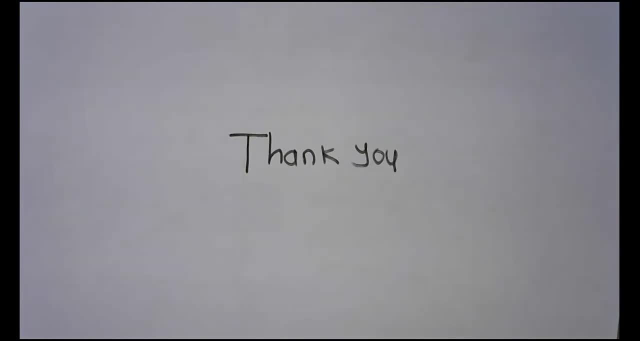 rate of reaction. We also tried to simplify it, simplify the equation to determine the finite change. We have also seen the graphical method by which, if the values of rate constant at different temperatures are given, then how, by graphical method, we can determine the value of activation energy. Now, in a simplified form or in an Arrhenius equation, if all except 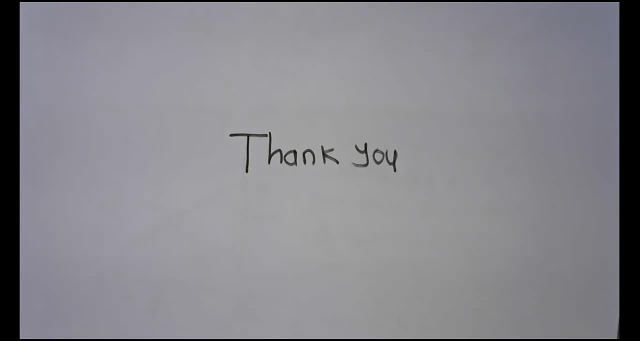 other variables are given, then the unknown can be determined. It may be that unknown to be determined may be an activation, energy, or it may be the value of rate constant. if the value of rate constant at one one temperature is given and if the reaction is to be carried out at another temperature. 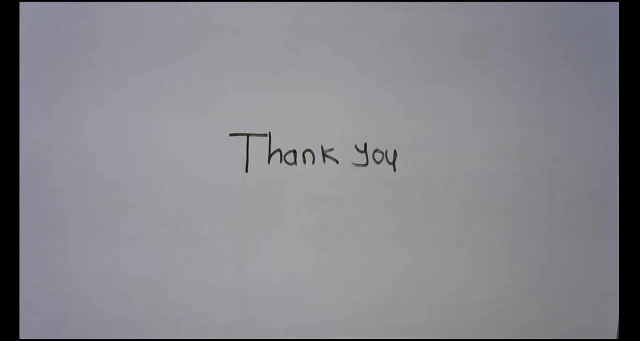 and if the activation is energy is known, then what would be the value of rate constant at temperature, T2? all this type of the calculations can be done using this Arrhenius equations, or say Arrhenius by using the Arrhenius mathematical expression of Arrhenius theory of temperature.